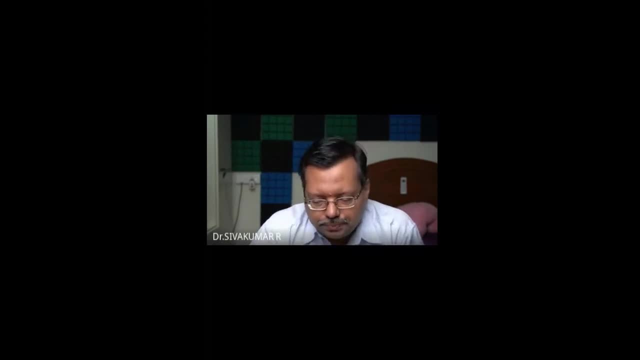 clarity should be there. Then it will be easier for you to move ahead. So whatever mechanics that you are actually learning in the BSc level will be called by the name Newtonian mechanics. Of course everything is Newtonian, But were we give some names so that you know whether you are? 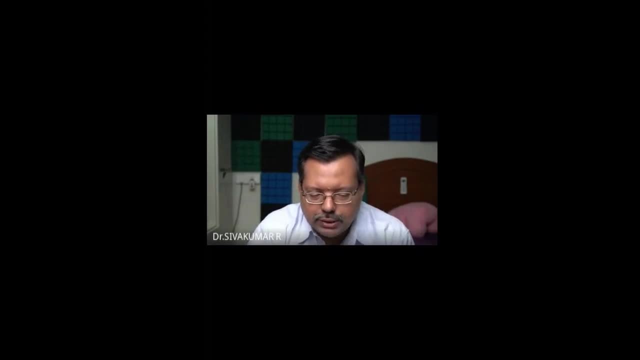 between the undergraduate mechanics or the postgraduate level. so for that reason it is traditional that people call by the name Newtonian mechanics for whatever you studied until your undergraduate course, so that that distinction is what I will tell you then, so that you will be knowing what is that. 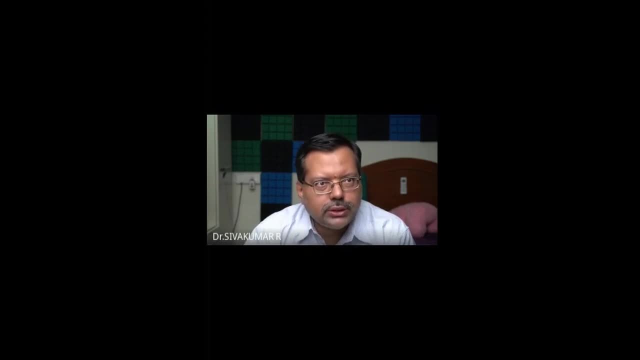 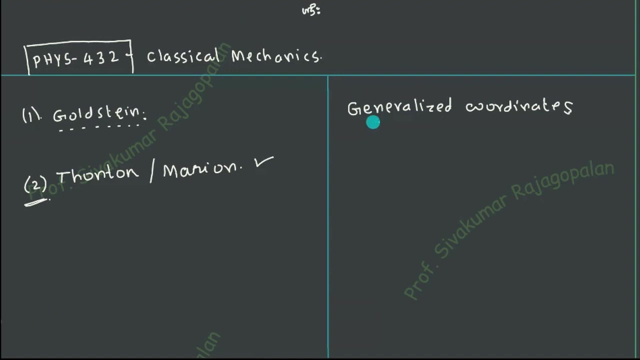 we are trying to do with the generalized coordinates, so I think that this cursor is not visible. I will bring the cursor. cursor is not there, okay, so that some kind of green color cursor will be there. no, okay, so here you can follow this cursor. so the first question is that what? what are you going to do with the? 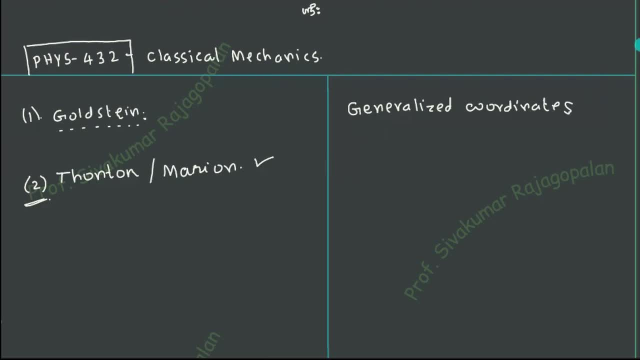 coordinates. that's what I am trying to say. so, when we are going to study the classical mechanics, the first point is that that we would like to know how much difference is when, compared to the Newtonian mechanics, we're going to make a transition to what is known as 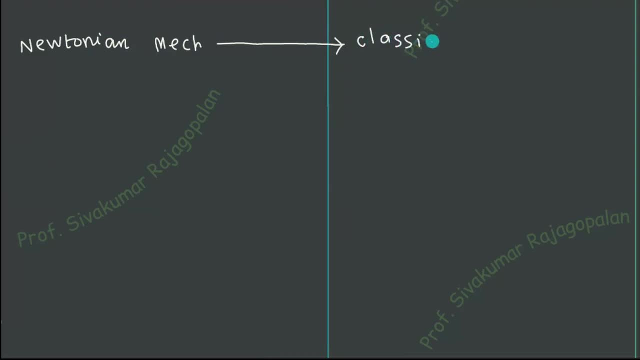 classical, so the terminology is like this. so the first course on mechanics is called a Newtonian mechanics, a second course on mechanics. Second course means you are reading mechanics for the second time during your educational system. So that is the reason and that is usually called a graduate level course. 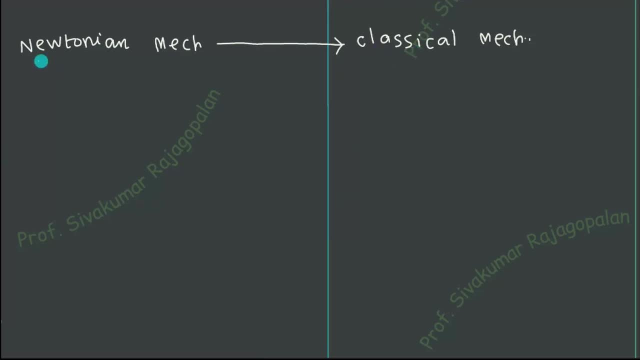 So graduate level course is known as the classical mechanics. undergraduate level course is Newtonian mechanics. That is how the terminology is designed. and why it is classical is that we are going to make further transition to quantum mechanics. So that is why the terminology is like this. 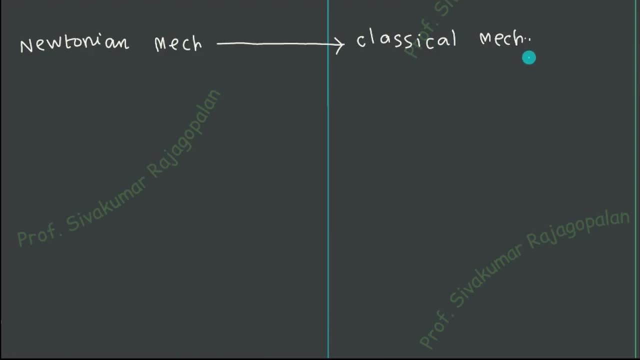 So from the classical we will be moving to the quantum and then of course there will be further. division will be there whether it is classical, relativistic quantum relativistic or non relativistic quantum. like that you can have multiple classifications. So when you see the name you will be able to understand what we are talking about. 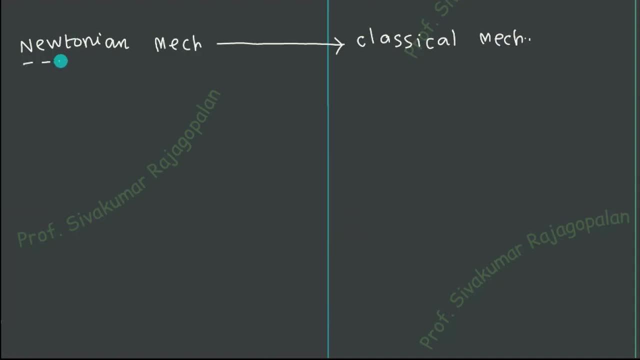 So that should be clear and what you generally deal. so what you generally deal in the case of the Newtonian mechanics is that you write down the traditional equation In this particular vector form: f is equal to m times a. This is how you write, because out of the three Newton's laws, only one of them is written. 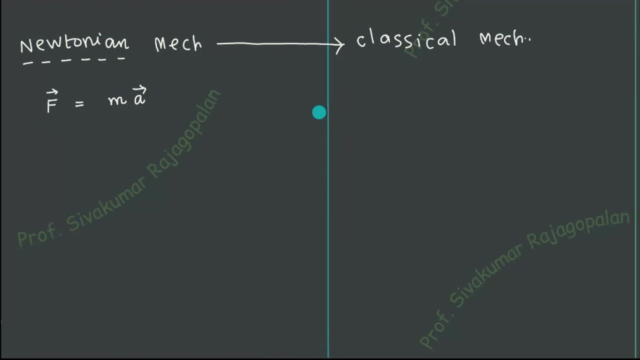 with an equation, The first equation and the third one. so we do not write it in the form of an equation, but it represents some information. So therefore we do not have equation for the first one and third one. Of course, third one is only equal and opposite, so we do not write explicitly that expression. 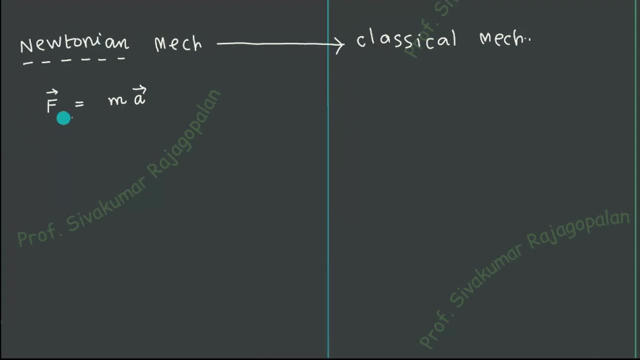 So the main equation coming into picture for the mechanics course Is f equal to m a. that is how you write and then you proceed further. in the case of the classical mechanics, we are not going to write the equation f equal to m? a. So that is the biggest difference. so there is a difference is there, and we are asking. 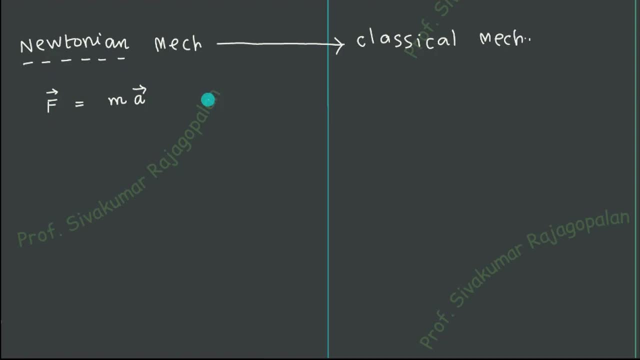 the question. some question will be there. what is that we are going to do with this? Now, in the case of the graduate level course, we are not going to write down f equal to m, a, but instead of writing that equation, okay, so let us come back to this discussion. 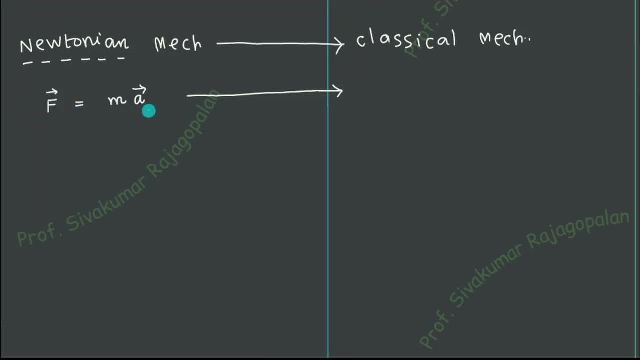 So We consider f equal to m a as a statement of what you call the observation. f equal to m a has come from observation, So Newton has done the experimental observations, and from the data he has written down this equation. that is how this equation has come. 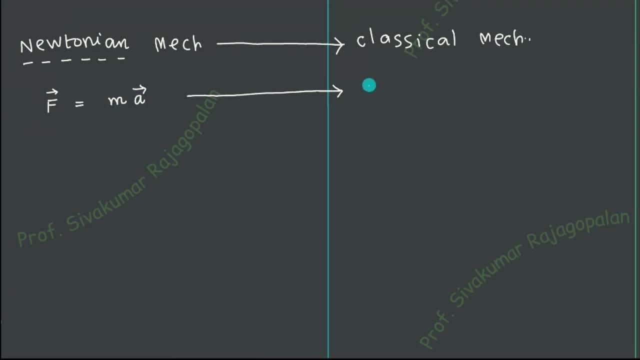 Now that we are, what we are going to ask is that in the graduate level course we ask the question why nature obeys Okay, An equation that looks like f equal to m, a. So that is a kind of a question that we are asking. we are not going to take that equation. 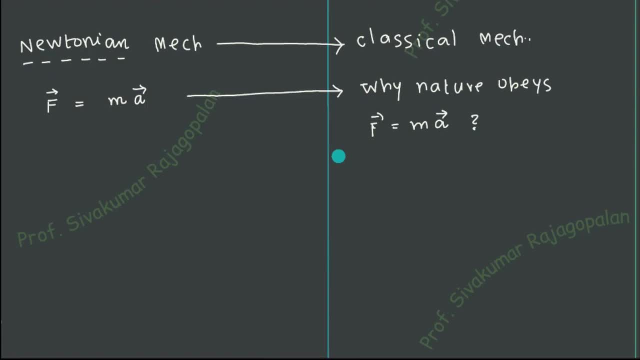 and then solve the problem that is already done. So we are not going in this particular semester. that is not the objective. So the main objective or the main aim of the study is very different. So in the UG course you start this particular equation. 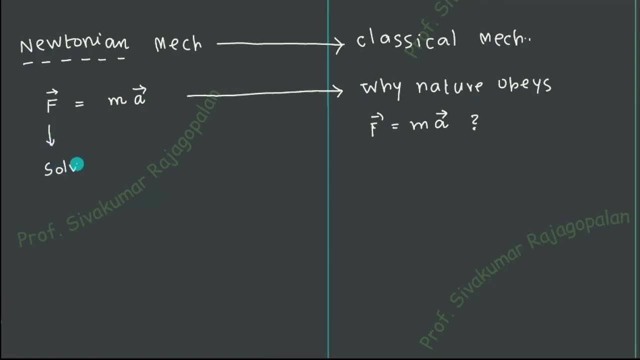 And then you start to solve the problem. Okay, That is the idea. And now here. the idea is like this: why the nature obeys such a such kind of some kind of equation? Let it be any equation. in our case, it happens to be f equal to m, a. 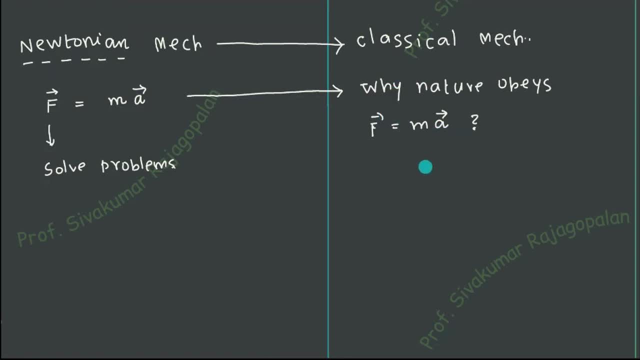 So we are asking the question: why should nature obey according to this particular equation? So that is the question and we are going to see a general answer. So is there any answer? really, is it possible to discover like that or not? So that was the objective. 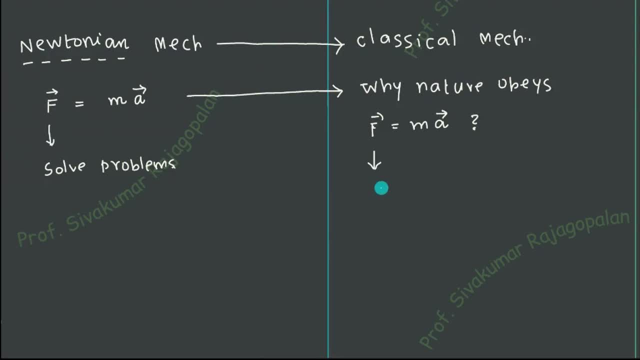 And the answer to this question is yes, people have discovered what is the reason, And that reason is answer is that it is based on the Hamilton's principle. So now you you started. what is the? what is the objective? The objective of the classical mechanics is to understand why there should be an equation. 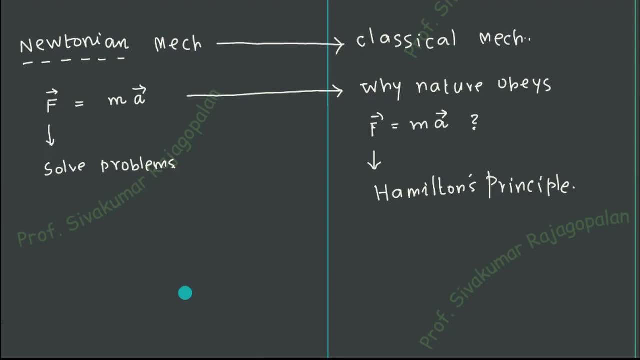 Okay, Okay. So the question is: why does it look like f equal to m? a? That is the question. Now, what is the answer to the question is the answer is this: The answer is discovered by Hamilton, And Hamilton has given a statement. 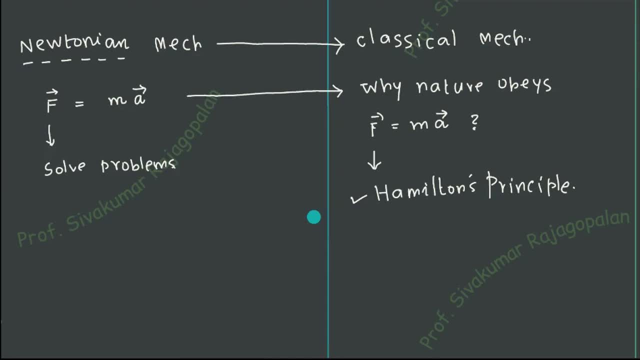 Now, that statement is what is known as the Hamilton's principle, And Hamilton says that, okay, according to this principle, everything in the nature obeys. That is the statement, And that everything happens to be f equal to m, a in the case of mechanics. 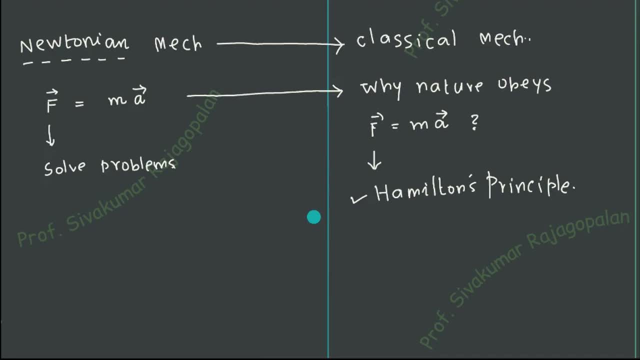 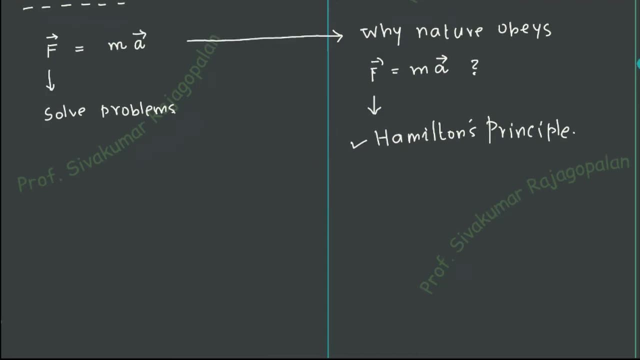 So Hamilton principle is a little more wider, it has a wider applicability than mechanics. okay, and to understand this better kind of understanding is: this is equivalent to: so i'll put three lines here: this is something equivalent to a principle that is already known to you generally, in optics i think. 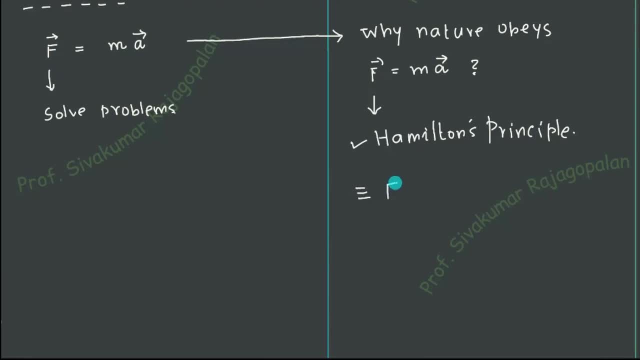 you must have studied in optics this principle, what is known as fermat's principle. why i am telling about the fermat principle is generally in optics people study. so that means you will have some idea about that principle and the hamilton's principle is going to be very 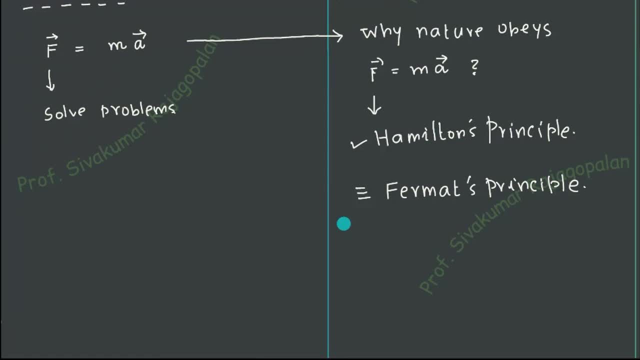 similar to that. so there is no big difference. whatever hamilton is going to tell in mechanics is what exactly is the statement in the case of optics? so small change is there in mechanics to optics. so that is the principle why i am telling about the fermat principle. 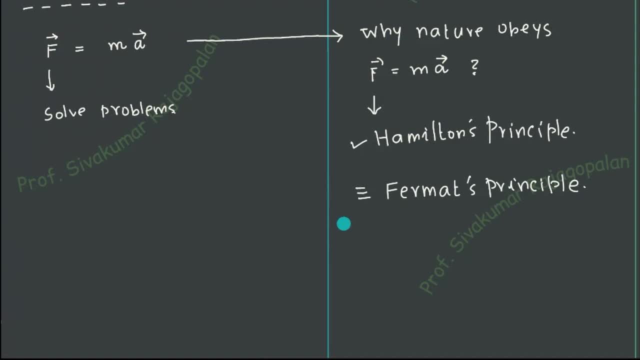 small change. because of that small change, the name of the principle is also simply changed. well, this is called hamilton's, that is called fermat's. and coming to the fermat's principle, because something you already know, in optics, i'll tell you what is that statement. if you take 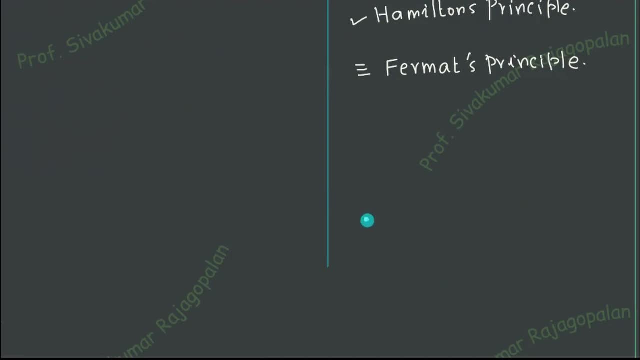 a particular light source, for example, and then suppose: if you are going to shine the light, for example, it's going to travel in a straight line, like this and it reaches to another point. so if you are going to shine the light, for example, it's going to travel in a straight line. 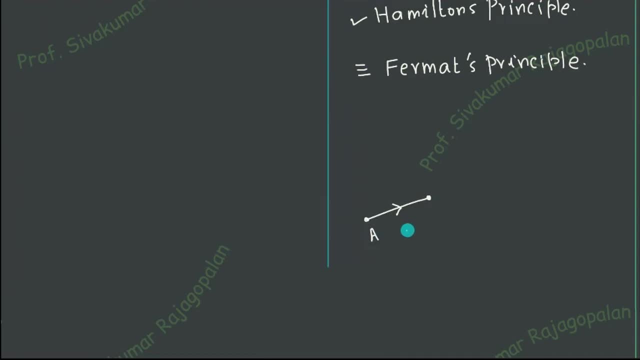 you are going to start the light source, like a torch light, for example, or a laser beam. if you switch on, then the light travels in straight line and reaches to another point, as long as you don't have some medium inside. if you are going to have some different, different material medium like glass, 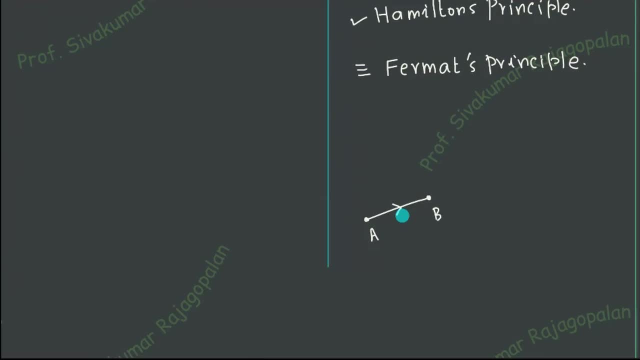 plastic and then some other transparent material, then followed by air, like that. if different materials are coming in between, then there will be bending of the ray, but if nothing is there, nothing is there means we are talking about vacuum. if nothing is there, then once you start the light, 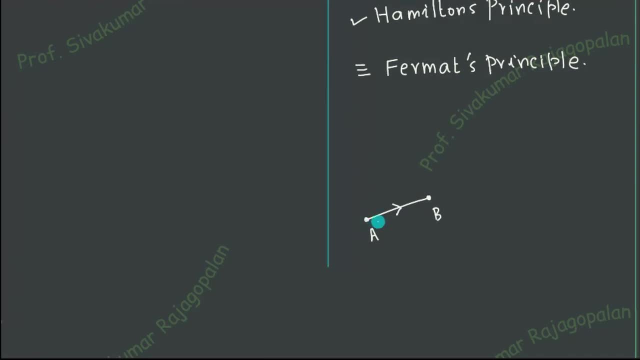 or that is called light source, is switching on, then the light will travel in a particular straight line and then reaches to the point b and because of this reason, the optics we usually called the ray optics. that is how you learn, first of all. so ray is actually a straight line. so once again, you 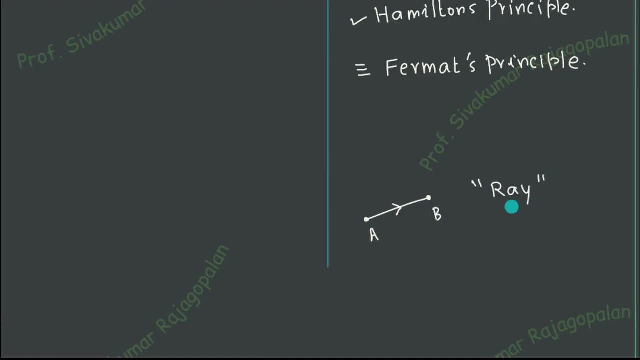 ask the question. what is the question is why light should travel in straight line. light actually can. light can travel like this. so if you are going to shine the light, for example, if you are going to shine this light this way, you can visualize like this and come like this. it can travel and come. 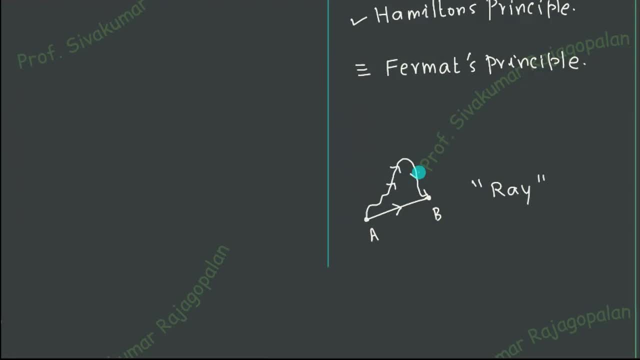 right. so why light did not go like that? so this is: this is not being observed in an experiment, whereas the straight line behavior is observed in an experiment. so we ask the question why? why straight line behavior is observed, why some other arbitrary path is not observed? that is: 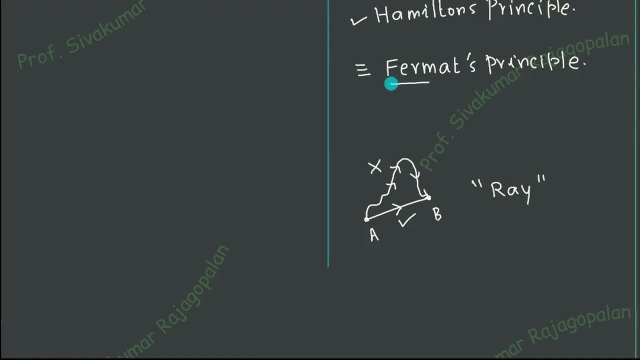 a question and the answer is fermat's principle. and fermat principle says that light way is different to what light went to the path that we will discuss soon. travel in that particular path for which the time becomes minimum. so that is how the statement comes. so this statement is familiar to use. okay, it doesn't tell. 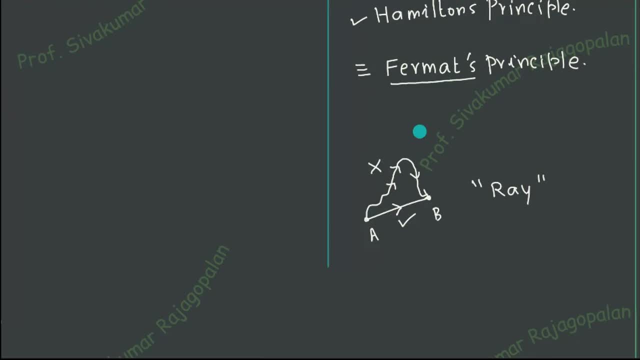 what is the structure of the path? but? but instead it gives you some kind of principle, what says that time is minimum, that is, time required to travel from one point to another point has to be a minimum. so this principle gives you the information about day. I'll write down that minimization of time. this is what 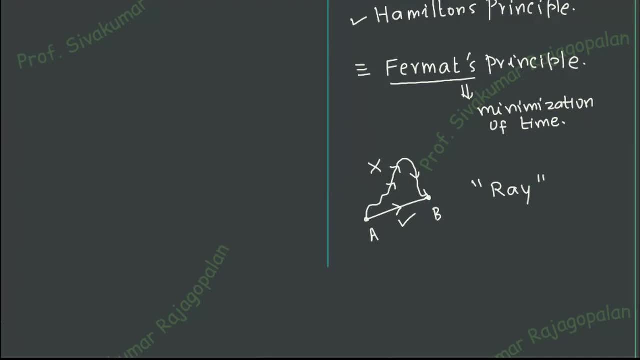 is taking place. okay, so anybody is joining. no, okay, fine, so you got the point. now the point is that the question is why light has to travel in straight line but not in either. the answer is there is some principle called a minimization of time, and that principle 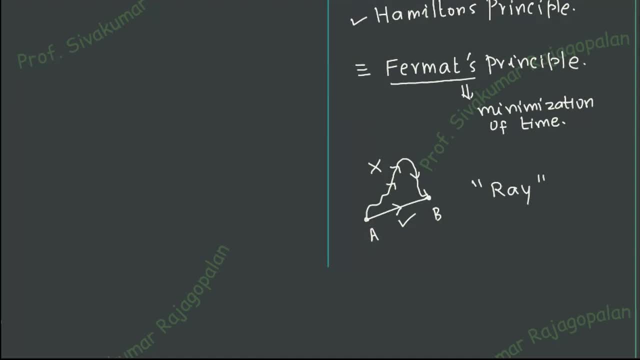 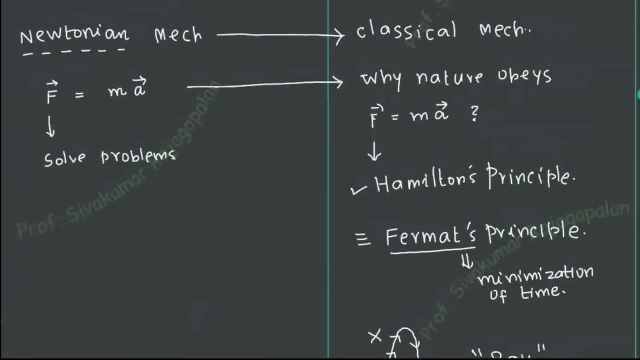 is called the Fermat principle and nature obeys this principle. that is the idea, and once this is clear to you, now we are ready to go back in the case of the mechanics. in the case of the mechanics, also, a very, very similar principle. okay, almost similar, there is no big difference, almost a similar. 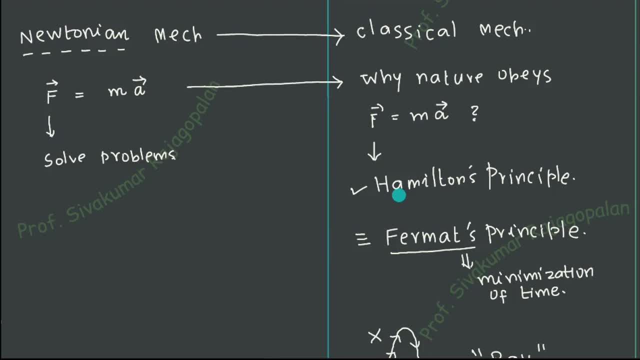 principle is going behind the scene. behind the scene means something that is not directly visible to you. what is directly visible to you is light is traveling in straight line. that is what is visible, but while it is traveling in straight line, that is not visible to you. so that is, that is the point which is coming as 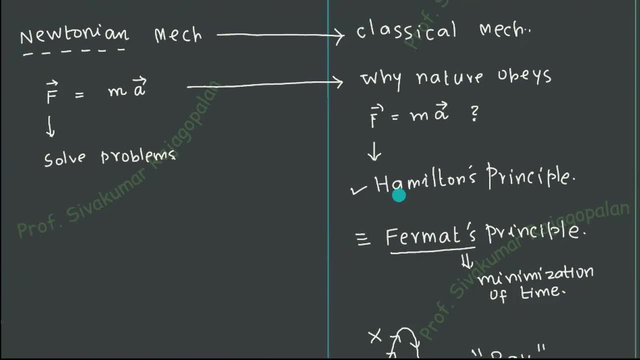 a principle. the principle is not directly visible to you. this has to be understood mathematically. so there is therefore: there is a, there is a. there is a big difference. now I will again come back here. in the case of the undergraduate course, you take the F equal to me and then start solving the 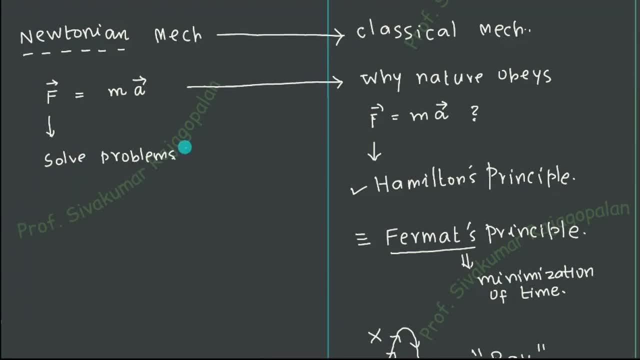 problems. that means you have to solve the problem. you have to solve the problem. that means you, you are going to consider some physical problems. like I'll say that this is physics. you, you take an example of an oscillator. you take an example of various pendulum. it could be compound pendulum, simple pendulum or 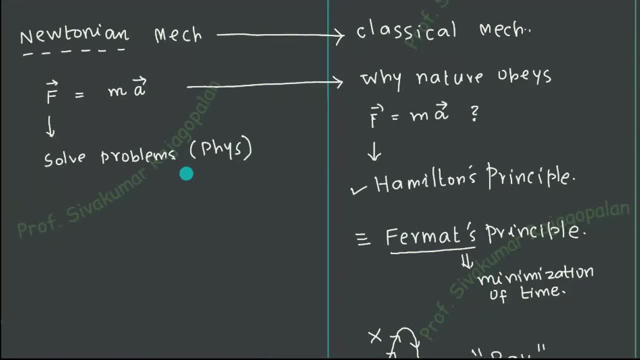 double pendulum, or horizontally oscillating oscillators, vertically oscillating oscillators, whatever we the pulley systems, okay, atwood machine like thing, anything you take, okay. these are the examples: considering the physical problems and then solving it. that's what we are going to do in the case of the 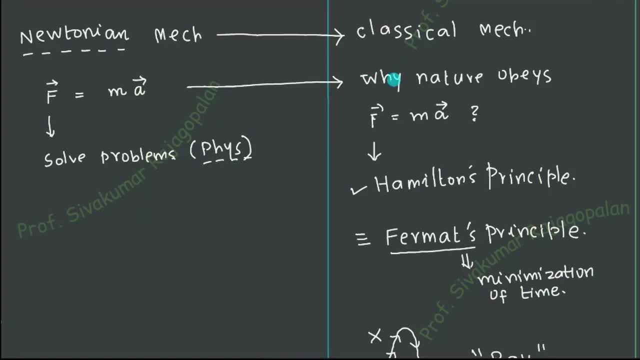 the điều, in the case of the innovative expertise and events were a big integral into solving these equations, which are proven. we have very well been doing before. how a? the particle of spectroscopy is visualizing theってIn the cases of the undergraduate course, in the case of 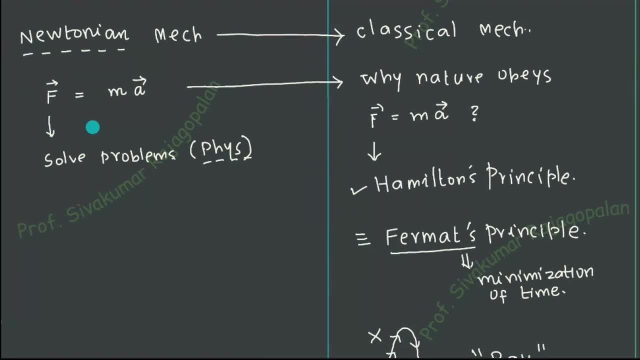 the classical mechanics. right now, what is happening is that this F, equal to me m, I'm followed to me feet 3.多 and, of course, here the point to be noted is that this is written down like m into x double dot, where you see that this is actually i am using the dot notation. x double dot means second time. 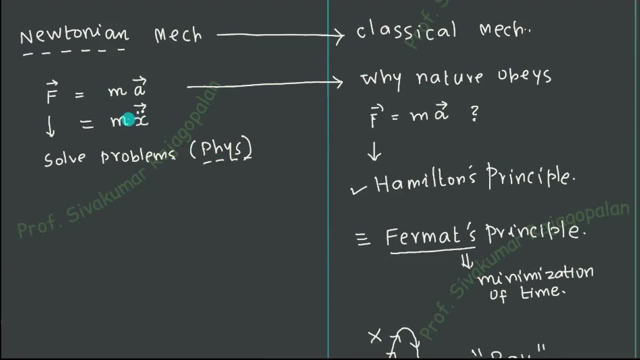 derivative of the position. that is how you write. so, naturally, what happens is there is a calculus is coming into picture and remember. once again, i do not know the exact year, but something like 1600. you know, newtonian period is something like 1600. that is the approximate time at that time. 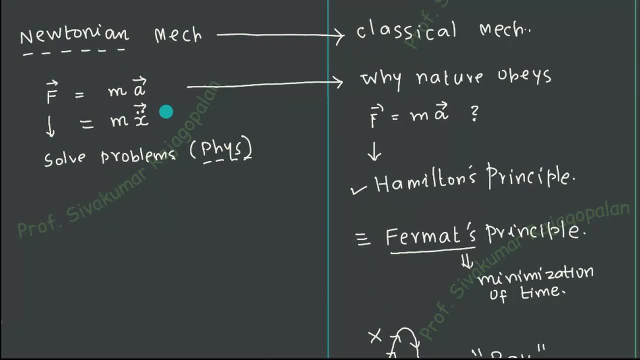 calculus itself was not there. nobody has discovered calculus, differentiation, integration, no one has discovered under such a situation. newton himself discovered the concept of the derivative. that point you should remember. so even though newton is doing experiment, being a physicist, he is the person who is inventing the concept of differentiation. 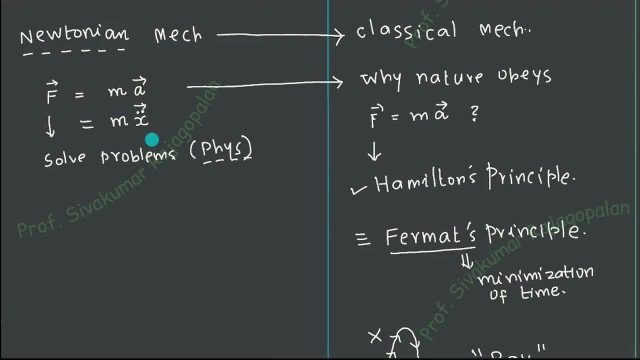 you know, and consequent upon that, parallelly, the mathematician who is the? i think lib, i think libnitz. right, libnitz is the person who has developed a more formal mathematical way of differentiation. so the idea of the derivative itself has come from the newton. remember that. 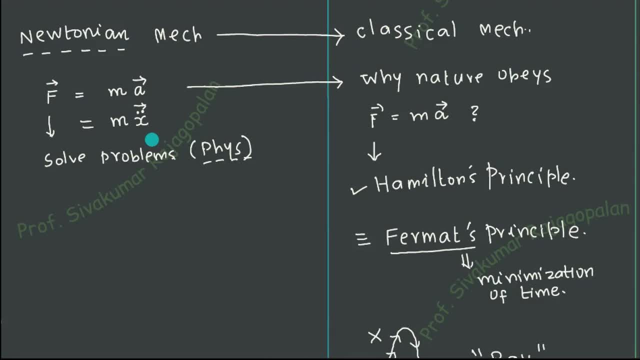 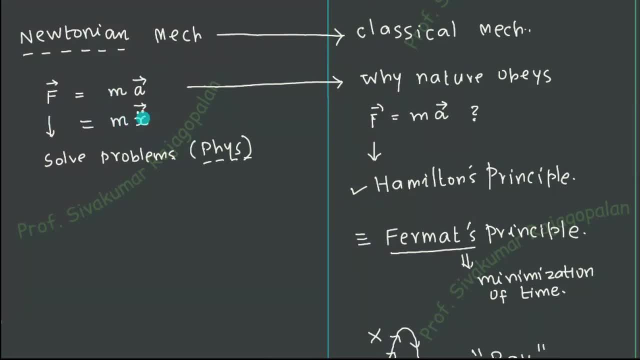 there are many formulas there, and now we have to remember that he, because of that calculus idea, only he, is able to write the experimental data into f equal to me, otherwise this equation will not come. people have to keep, or we have to keep, only the numbers. that's all. several pages of numbers will. 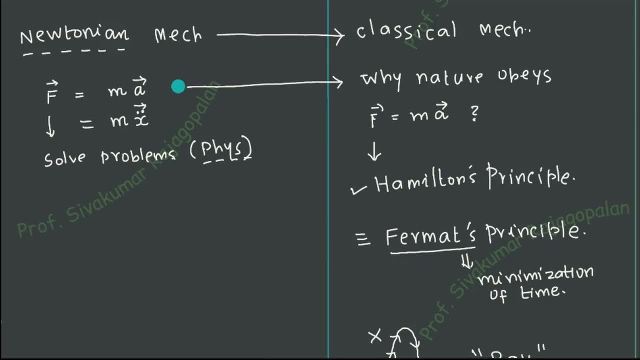 be there. okay, how to rewrite this entire set of data, that is, numbers, in a particular equation that has come only from the concept of the derivative, which he himself discovered sometime in 1600. okay, 1600 is easy to remember exact years we will not worry about. okay, now the question is this: now, the question is that this: 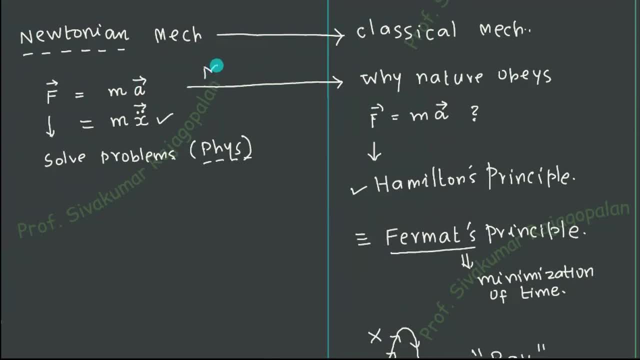 being the experimental evidence. we are asking, uh, more more fundamental. more fundamental means, remember it is more mathematical, so i'll write down that. so we are. we are moving from the physical aspects of mechanics to the mathematical aspect of mechanics. this is very important. so you ask the question: what is the big difference between the bsc level mechanics and the msc level? 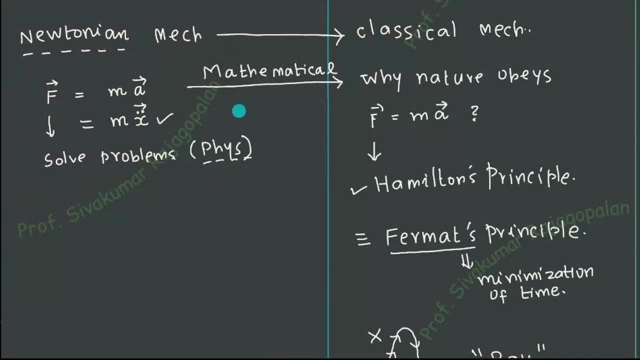 mechanics. the answer is bsc level. mechanics deals with experimental uh, experimental data and mostly physical systems. that means systems that are uh that can be done in a laboratory. that is the bsc level. coming to the msc level means we are going to ask more fundamental question: what is that? 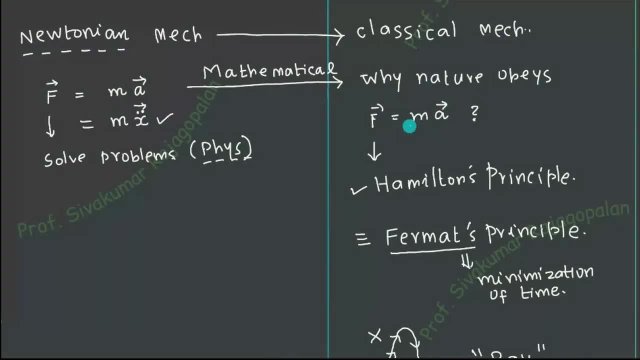 question here. it is there: why natural base? that's a fundamental question. so to get the answer to this question, we cannot do any experiment, so the answer lies in mathematics, not in physics. therefore, now, this is- this word is important- mathematical. so classical mechanics. what is classical mechanics is classical mechanics is. 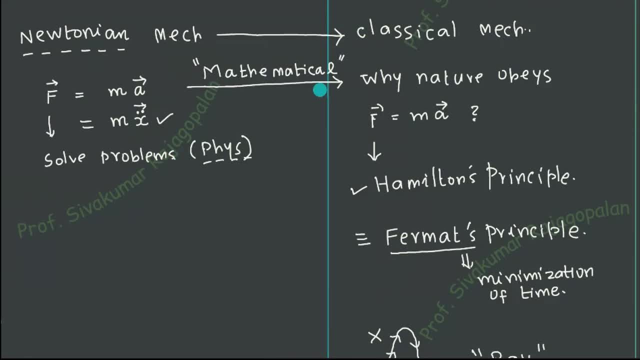 understanding mechanics using mathematics. so that is the correct way of understanding. define classical mechanics means what classical mechanics is. understanding mechanics using mathematics, and therefore classical mechanics, is nothing, but it is a way of studying mathematics. so this is a very crucial concept. that should be clear to you. that, essentially, whatever we are going, 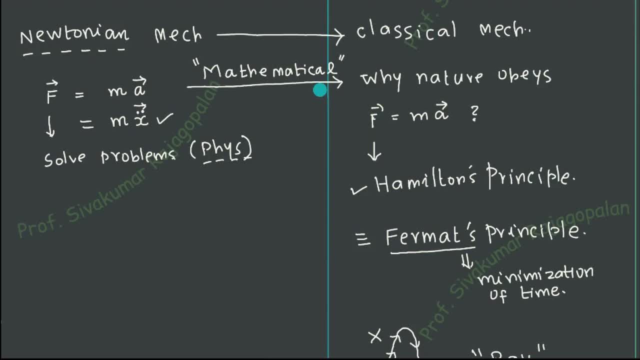 to study in this particular semester on the classical mechanics is nothing but is nothing but mathematics, okay, so that point should be clear, okay, once again, you should not think that, okay, some experiment is there, some pendulum is oscillating. we are not asking about any experiment. nothing will be there in classical mechanics, so it's all about understanding their nature. 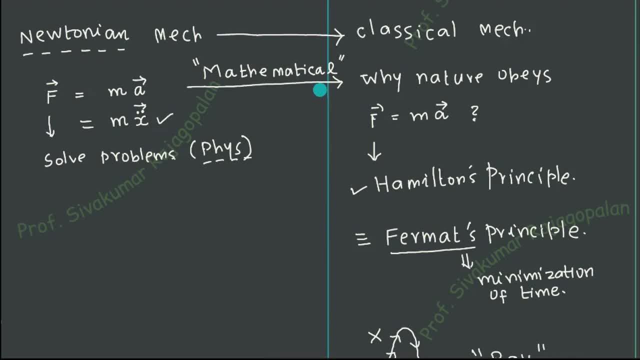 using the language of mathematics, so that this is something which is important, because the starting of the msc level, generally msc level, is: uh, overall structure will be like this: uh, in the case of quantum mechanics also, same same idea is same. so in the case of quantum mechanics, uh, we will be having a similar. 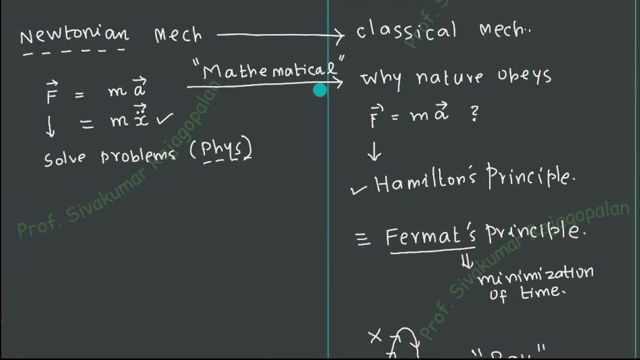 situation. you studied the photoelectric effect. uh, you studied the davis and jeremy experiment. everything is experiment. you got the evidences. electron can behave like particle. that's what i instantly did. right, quantum, quantum theory of the aircraft. but however, uh, davis and jeremy experiment has given the 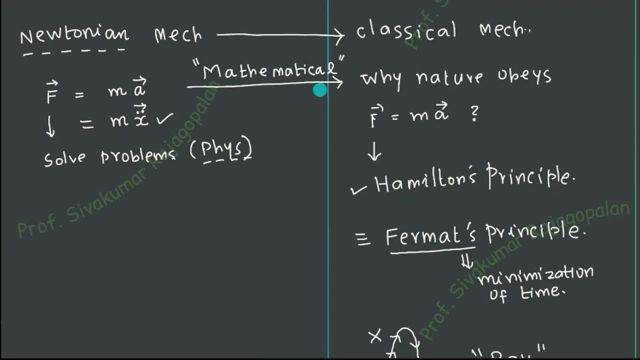 idea that electron behaves like wave. so whether einstein is correct or whether davision is correct, that is the question. both of them got the noble prices right, so you can't say one is wrong, the r, and other is right, so ultimately both of them are physicists. they, we have the experiment, but however, 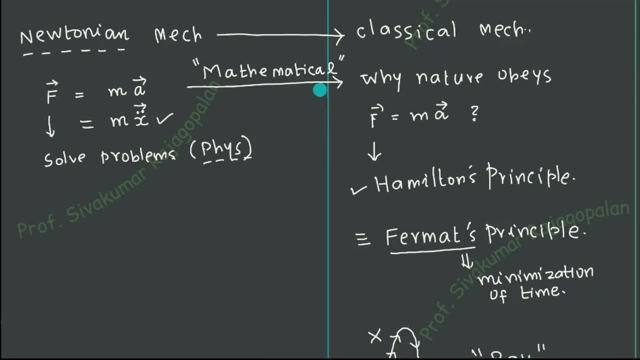 so at this particular question, when you are asking the question, then the study becomes mathematical in nature. so you understand the transition from physics to mathematics. physics means doing an experiment and then collecting the data. that's physics. and after that you got the data. okay, davison germer experiment. i have the data. photoelectric. 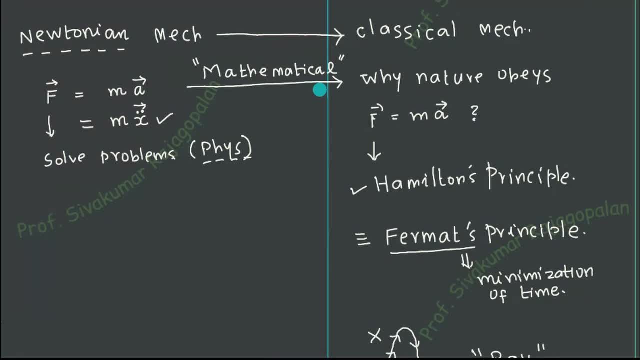 effect. i have done the experiment and got the data, but i don't know why it happens, why it is behaving like that, why electron is behaving like that. i don't have the answer. if you want to answer, you have to make a transition to mathematics. you can't get the answer in physics. 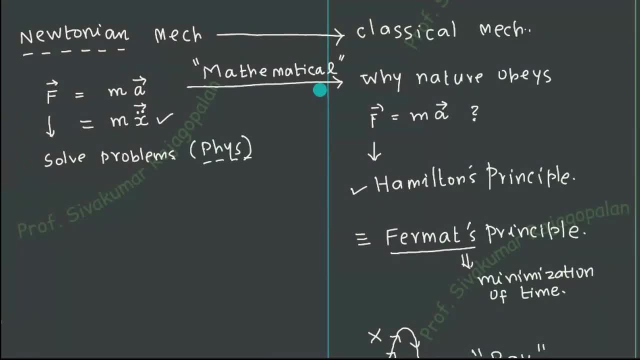 that is a place where we are going to make a transition. now. that transition is the bsc to msc transition. in the bsc you study the more most of the time, you study the experimental observations most of the time and in the case of the msc or we try to understand why nature 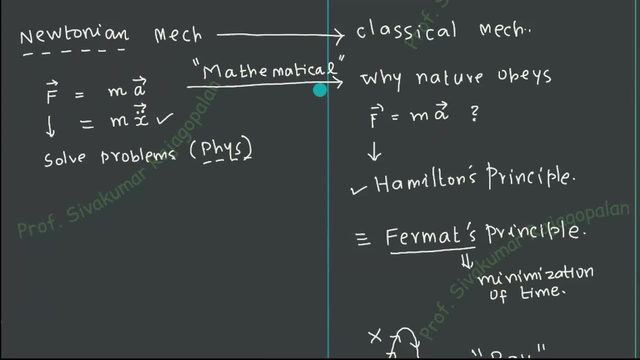 behaves like that and therefore it becomes mathematical in nature. so quantum mechanics is nothing but mathematics, classical mechanics also, same. and we are of course later we are going to study the statistical mechanics once again. statistical mechanics is nothing but mathematics. mathematics of what? mathematics of thermodynamics. so mathematics of thermodynamics is the statistical mechanics. so ultimately this: 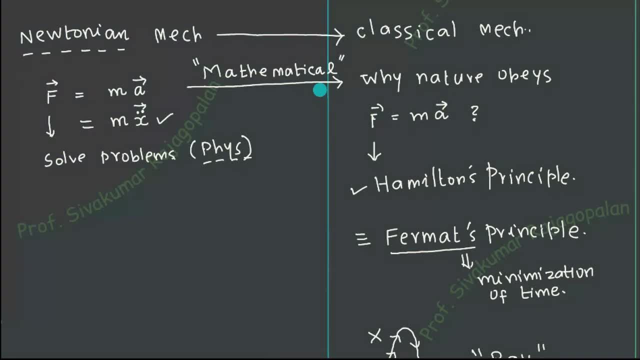 is the overall overall idea you should have. overall idea is that the two year msc program will be will be mathematical in nature and this is what people say theoretical, so theoretical physics. so what do you mean by theoretical physics? is theoretical physics means a physics wherein you 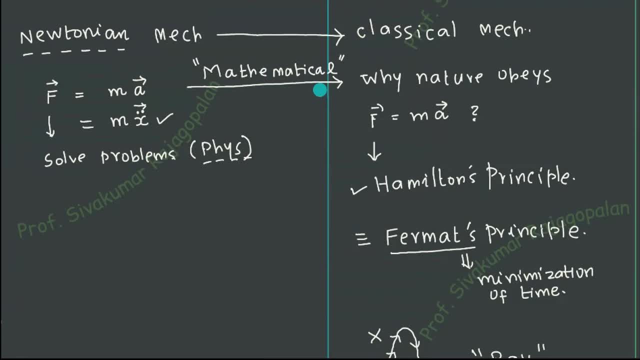 try to use mathematics to understand. okay, so that is the overall idea. so do you? i think you are following. you have some general questions, something like that you can ask. okay, then we will proceed further. yeah, anything, any any questions that you want to ask? hello, no, sir, we'll continue okay. 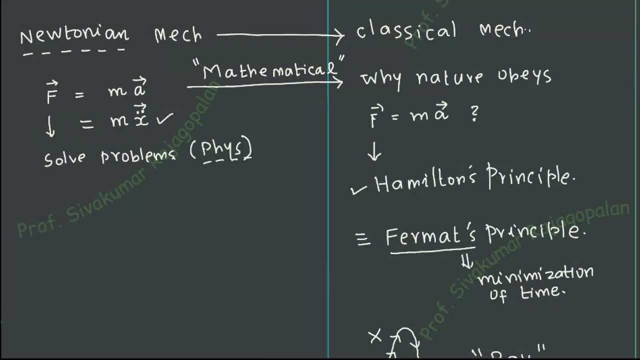 sometimes. okay, that's fine, we can continue. so if you have some general questions, you can ask me in the comment section below. so if you have some general questions, question in between, you can also ask this. okay, fine, okay, so now. so this is now the overall overall picture should be clear. okay, the the main. there is a big difference between the. 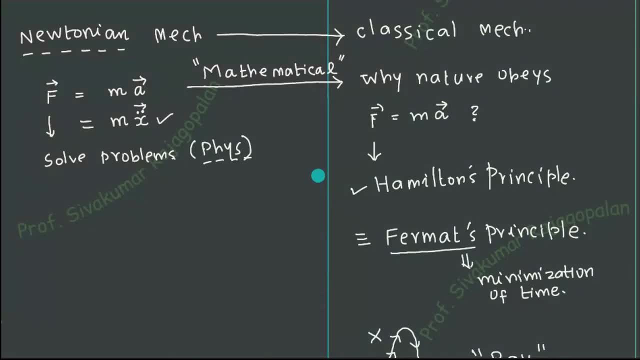 the ug study and the pgi study and the current msc level program, whether it is classical mechanics, quantum mechanics, statistical methods or the solid state physics- anything that you take, yes, it will be, uh, it will be. using mathematics, we are trying to understand the physics and the 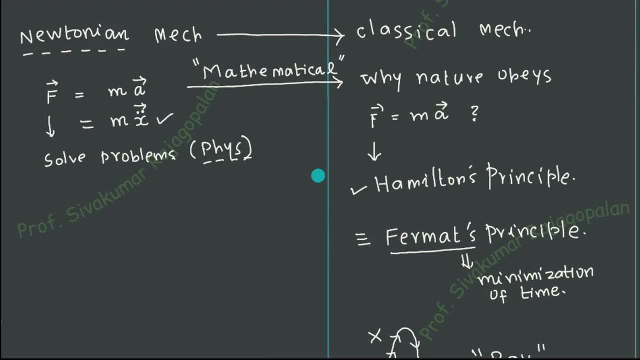 therefore, and therefore it is called theoretical physics- you will be doing experiment. of course, there is a different thing: learning. the experiment is also there, in the form of laboratory, but but as far as papers, theoretical papers- are concerned, the main thing will be mathematics and therefore, because of this reason, what I am trying to say is: you have to pay more. 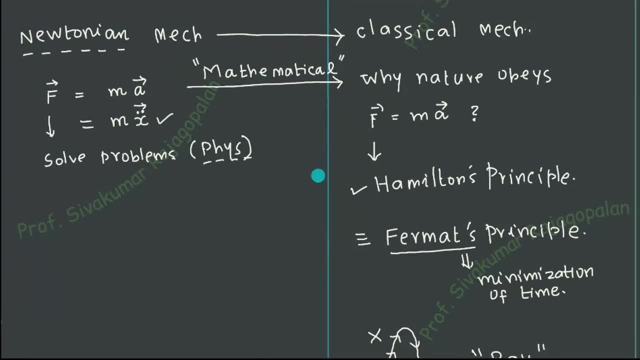 and more attention to learn the various topics in mathematics. now this point is very important. okay, the general idea that mathematics you know you can keep it to a minimum level, such as ancillary mathematics, allied mathematics, that kind of you know. reducing the level of mathematics is not a good idea. so try to focus more in, try to give more attention to learn. 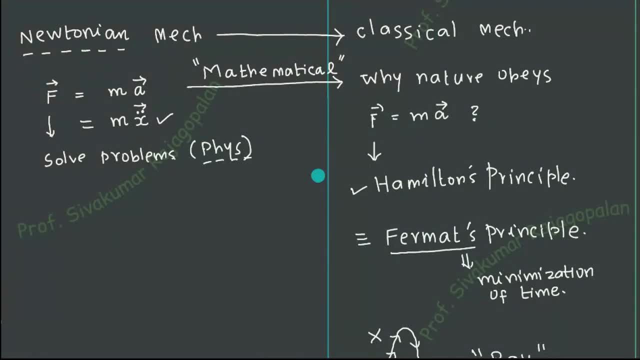 various topics in mathematics. okay, so the more and more you learn mathematics, the better and the better you can understand the physics. this is important. doing experiment- experiment is only a kind of skill. okay, you will be developing some skill in doing experiment, that's all about it. but when it comes to understanding, okay, experiments may not help much experiment. 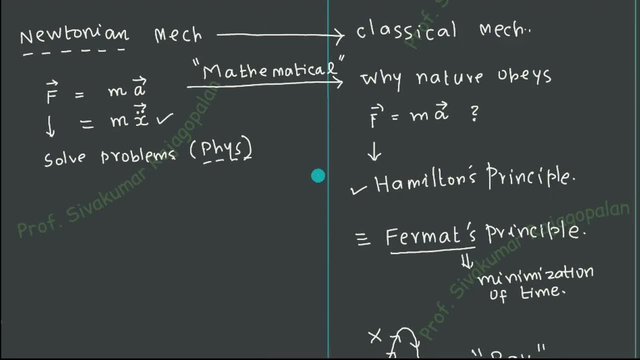 is actually a kind of a skill. okay, you will be developing variety of ability to perform certain experiment, that is. that's a different story, actually, and understanding is a different story. so these two things are two different streamlines. because of this reason, you should remember, because of this reason, after finishing your master degree, when you are going to perform, 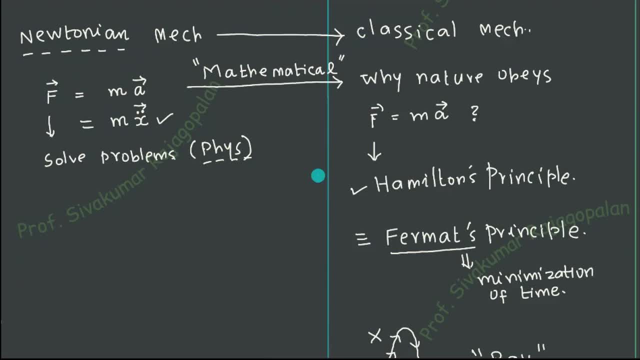 a doctorate degree. the first question that people ask is: are you interested in doing experiment or are you interested in doing theoretical physics? so that question is a very first question that people ask when you finish your msc course. so therefore, you should be clear about that, okay it. 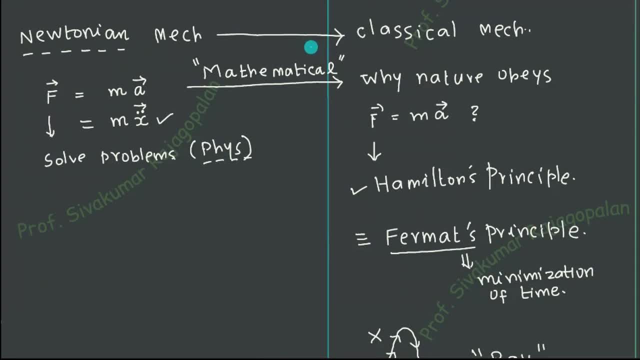 all depends on how much mathematics that you are math about that, okay. so after doing your master degree, going to learn from your side. that is there. so, of course, for the, for the sake of understanding mathematics, we will be having two papers on mathematical physics in our, of course, in our. 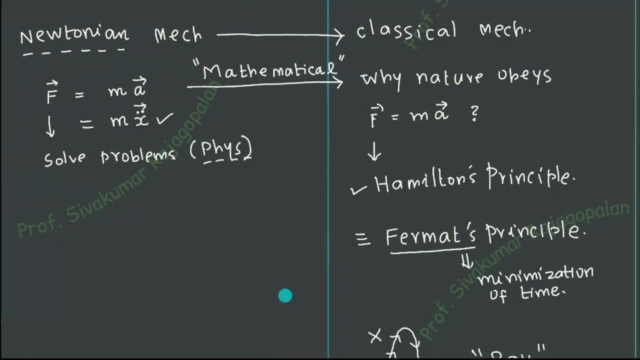 department. the first paper will be primarily focused on the differential equation and complex variable. that is the first paper overall. that is, these are the two topics. the second paper will will be generally, will be generally discussing about the abstract algebra, linear algebra and then group theory. that will be the second paper on mathematics. so these two papers will generally 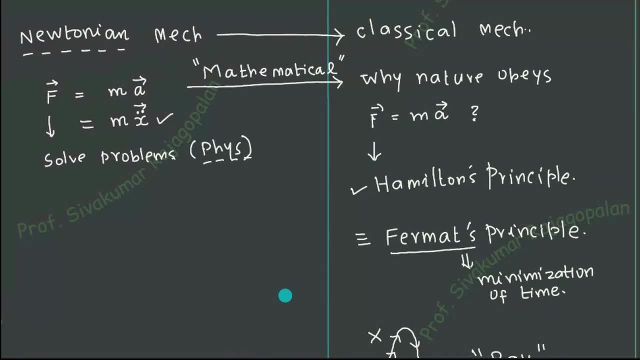 give you a good idea about where to start and then read. so. so the point that i am trying to say is that try to give importance to the all topics and mathematics. that's very much required. okay, fine, that's fine. and then, coming back to our problem here, 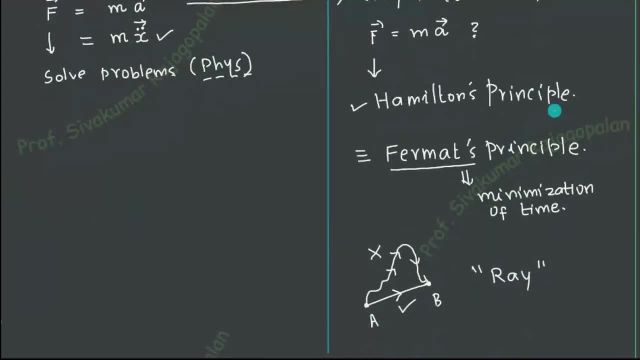 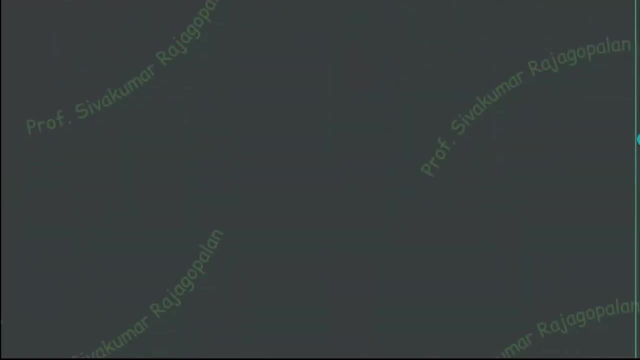 yeah, so now we are coming to the question on the hamilton's principle. so the hamilton's principle is going to be very similar to the fermat's principle. okay for match point, where i already explained. okay with respect to the time. so in the case of the hamilton's principle, is that, instead of time, it is something. 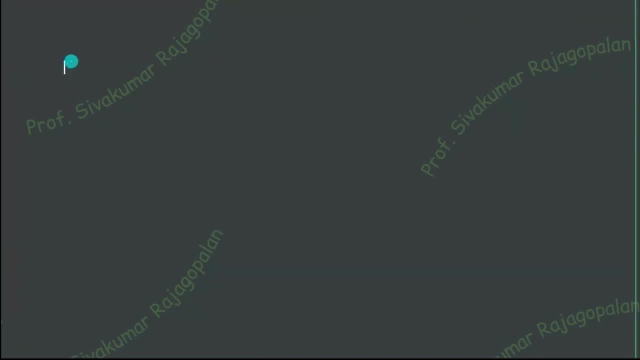 slightly different. so i'll now write down that, in the case of the hamilton's principle, the time taken with respect to the time taken is different. there is a small difference between the two principles, and the difference is this. so this is the minimization of of the hamiltons principle. now, what is that? something is that is called action, so it is. 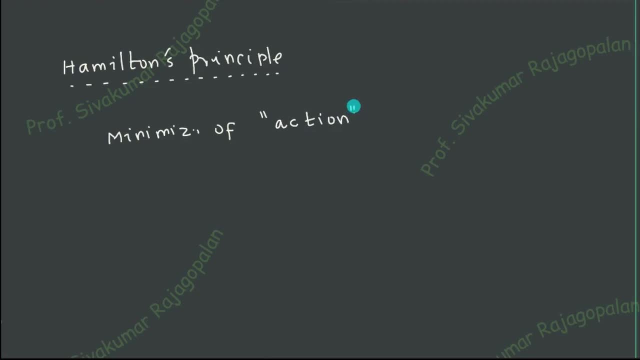 just given a name, that's all. no need to worry about the terminology. so it is not time now. time is not minimized, distance is not minimized. it is neither time nor distance, so it is something different. so therefore, we have to give some name for that. okay, so that's all about it. 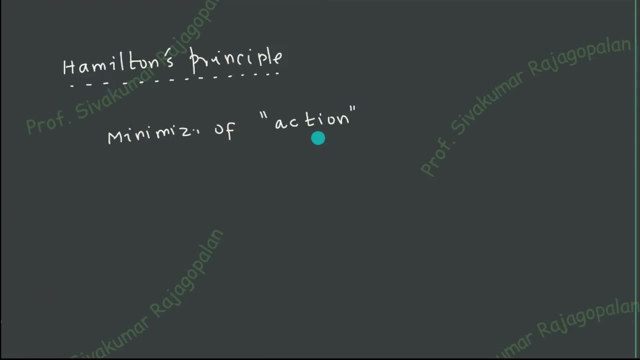 and people have given the name action. action is minimized if you say that a total money. if i tell in terms of money, for example, you can easily understand: uh, if you are going to get some, let us say you get a salary. okay, today is the first of the month. okay, when the first of the 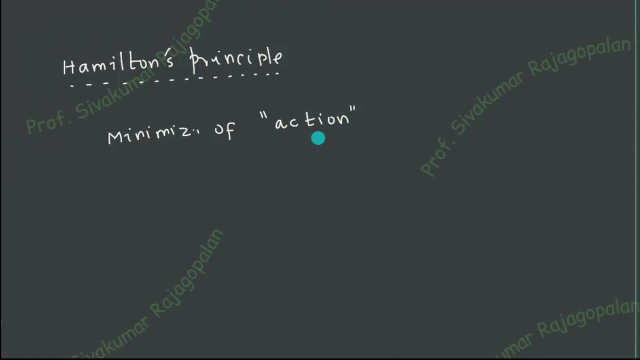 month comes. okay, you get the salary, and okay, now, what is your objective? what do you want to do? so, uh, we want to spend the money, right? so the question is that, when you want to spend the money, how do you want to spend? do you want to spend a lot of money, or that you want to minimize? 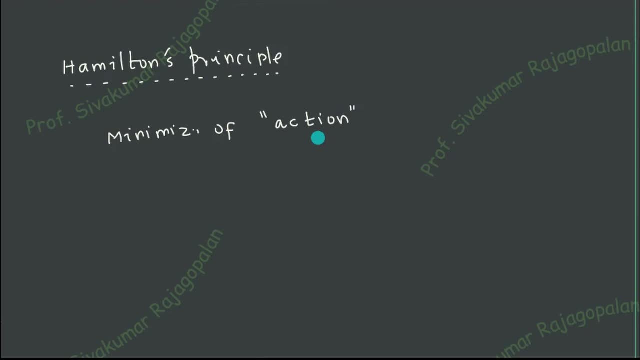 whenever you want to purchase some item, you will always compare: uh, what is the price in shop and then see who is selling it- minimum rate- and then you purchase from that right. so what is going on in your mind? in your mind, you are, there is something going on, namely that i have to spend minimum. 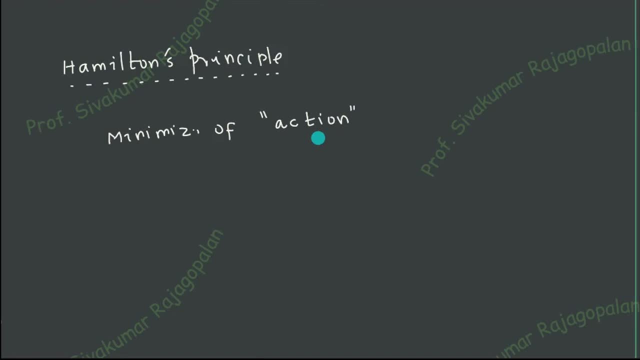 money. so there is a minimization, so give the importance the word minimization. minimization will be there everywhere, whether it is physics or not. everywhere this minimization is going on, it will is, it is there without even, uh, you realizing. you may not realize it, but it. 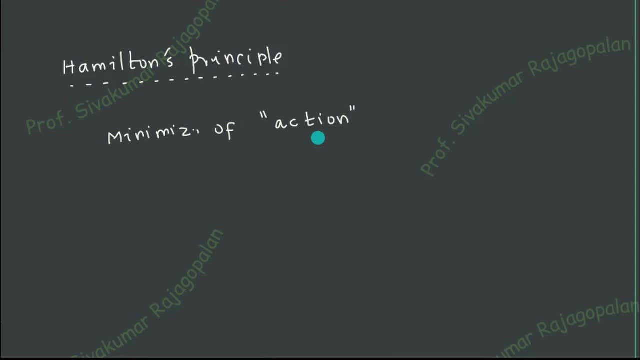 is an everyday action right. so it is an everyday action, right. that is the reason why the word action is there. minimization of action. what is that action? action means, what is that your? it depends on. it depends on place to place. the action will change in the case of spending the money. it becomes. 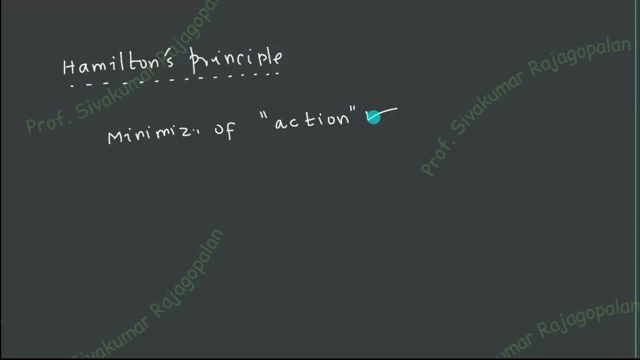 minimization of the money. now. forget about, uh, spending the money now. you are not. you are not getting the salary right now. you are a student. so, after finishing this msc, what do you want to do means you want to get a job. so when you are going to select the job, what will you do? do you want to go? 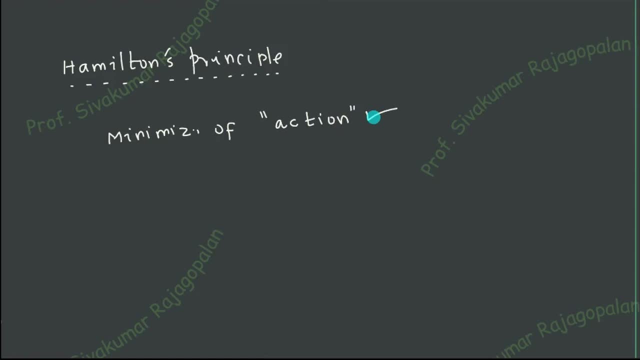 for a company who is giving minimum salary. at that time will you do the minimization. yeah, no right. what will you do? you do a maximization. so out of the four companies, or five companies, you will select only that company which gives you maximum salary. so what is going on is maximization is going on. so 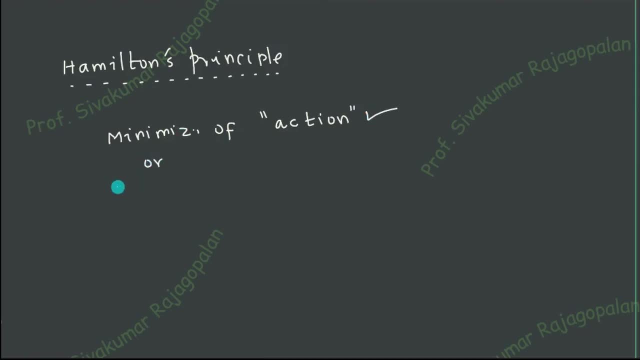 therefore, this word is very important. this either minimization or maximization either, and either this or that will go on. it will be there everywhere in the life. this is what is known as the principle. so now we will come back. come to this word here: principle. principle is applicable to a wide variety, not a small. 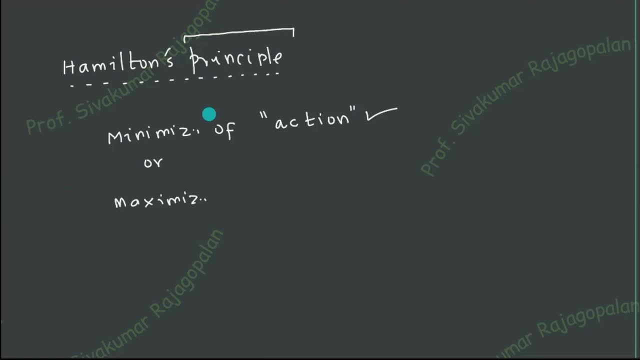 one. it is applicable all around. okay, Hamilton's principle is going to talk about either minimization or maximization, you, so I'll put a box here and then I'll say that this kind of wording is now coming here. right, what you call the minimization or maximization now instead. 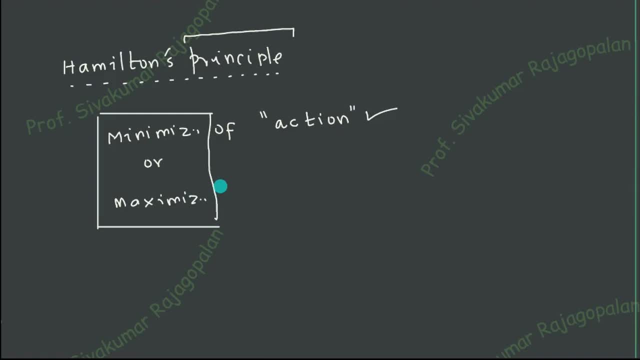 of saying two English words: minimization. one English word, maximization, second one. I don't want to use two English word, so combine them. if you combine them, this is known as extremum. so we say that this is an extremum principle. so what is meant by extremum is. extremum is either either means it can be minimum, 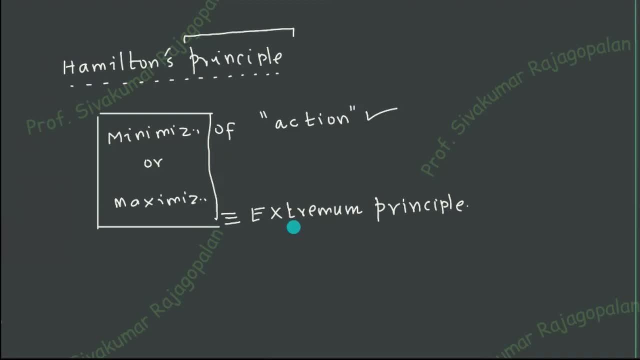 it can be maximum, depending on case by case. in one case it may be minimum, in another case it may be maximum. so that is a general term. so now you understand what is the meaning. so now you ask the question: Hamilton principle is minimum, minimization principle or maximization principle? that is a question. answer is: 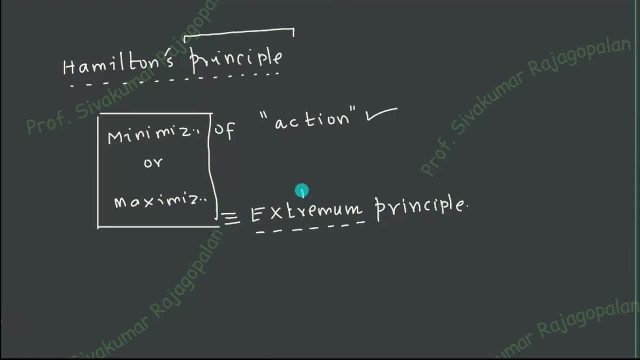 it is either way. so we say that hamilton's principle is an extreme, is a principle. extremization means either minimization or maximization, depending on a particular system, case by case. we can't say that everything will go along minimum, everything will go maximum. no, in one case it will be this way or another. 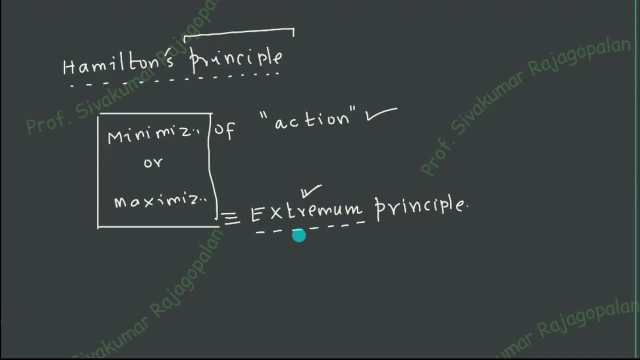 case, it will be that way. take an example of auto driver. if you take, you come to the bus stand. for example, you come to Pondicherry and take a auto and say that I want to go to Pondicherry University and the driver will go in all of small. 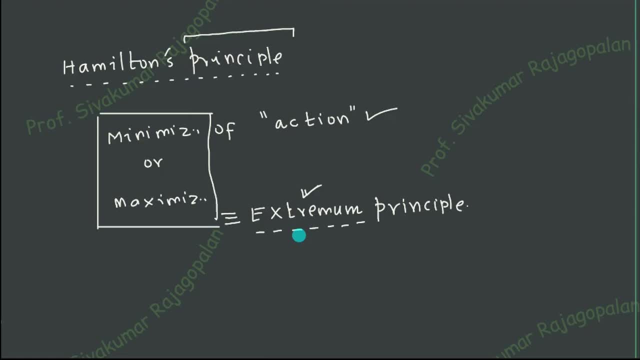 small streets. okay, he won't come in your main road, right? then you will ask the question so you can go through main road, right, why he has to travel in small, small road. then you ask the question to the driver- I mean auto driver. you know the answer, right? what is the answer? he will say that I want to minimize the. 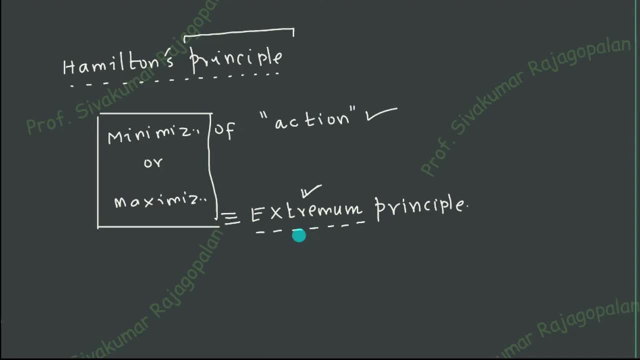 petrol, isn't it so? so what do you understand? is that minimizing petrol means once again coming back here. so I am trying to give some possible situations where your your not only in physics, actually okay, it's all about nature. everywhere it works, and therefore the principle is known as the extremization principle, as an Hamilton. 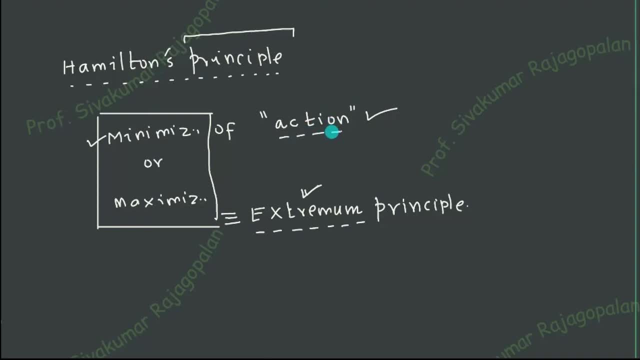 principle, and that is what is the action. action means what people do. people behave different way, people behave differently, differently in different situation, so that is known as the action. so now, in the case of the hamilton's principle, we are asking the question: what is the action for the hamilton's principle? 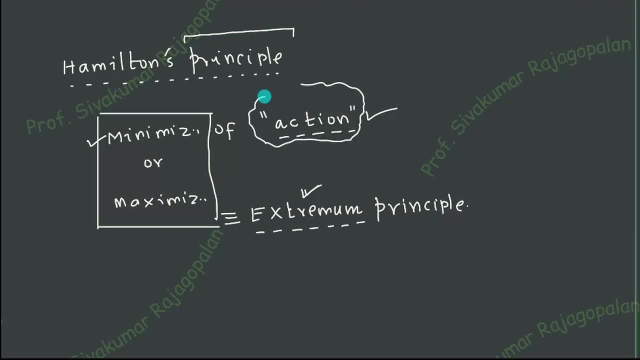 so that's that i will write down now. so in the case of the, exactly for the case of the hamilton's principle, this action is given by this integral, the lagrangian multiplied by the dt. that's all. so now you can understand what is happening here. in the case of, in the case of the, you know, 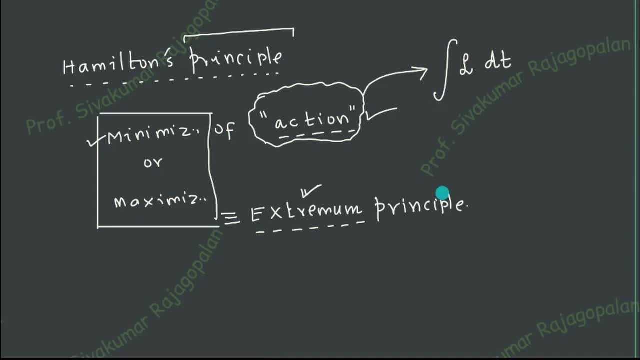 comes to the money or it comes to the minimization of the petrol. we use the word money, we use the word petrol. so these are the english words that we use to find. and in the case of the fermat's principle, you say time, time is minimized. you say: that looks very simple. you simply write down time. 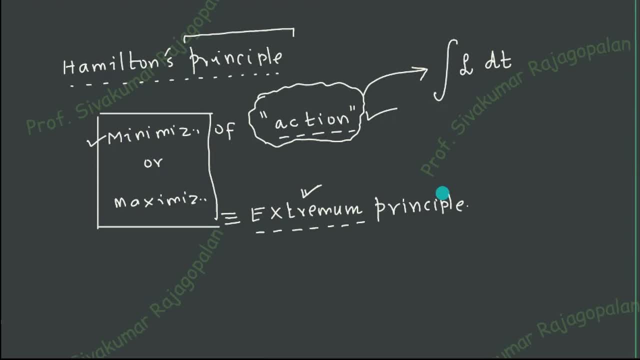 but in mechanics what happens is, it is not a simple quantity that is getting minimized. if it is very simple, we can write down space time, something like that. we can write energy, for example. it is not that simple quantity. it is a quantity that has to be evaluated according to this rule. you evaluate this quantity integral of. 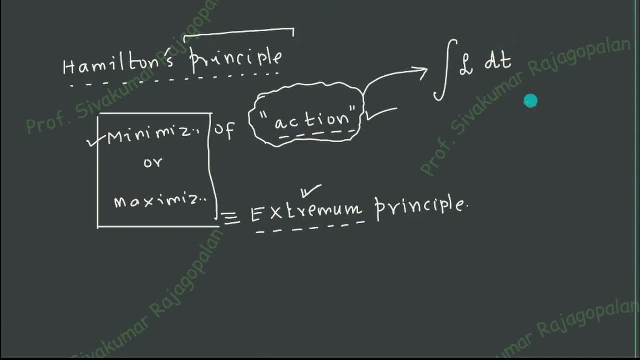 lagrangian multiplied by dt. you evaluate: okay, whatever it is, you call it by a. so whatever comes as an answer that you give the name a, that a is known as action. now this action has to be minimized or, in general, it is okay, minimized or maximized, but in majority of the system. 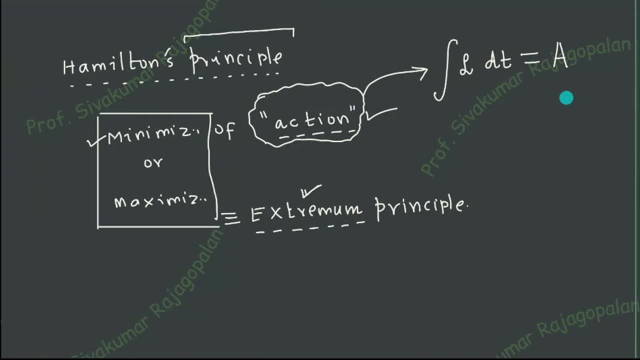 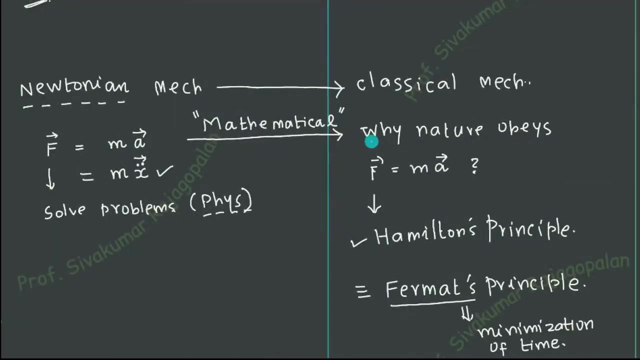 minimization works in mechanics. so this is the idea. so now you got the overall idea. so, uh, what is the question and what is the answer? you should know, uh, of course, let me go back in the screen and see the question here. the question is this: here it is. the question is this one, why nature obeys f equal to ma it has. 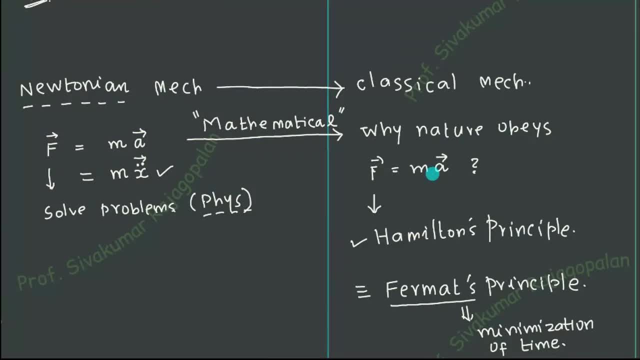 why nature should obey an equation of the form. it need not be if equal to me, whatever it is. that's that's the meaning. whatever be the equation that is currently obeyed according to the Newton, nature has to obey according to that. that is the question. the answer is that because nature is 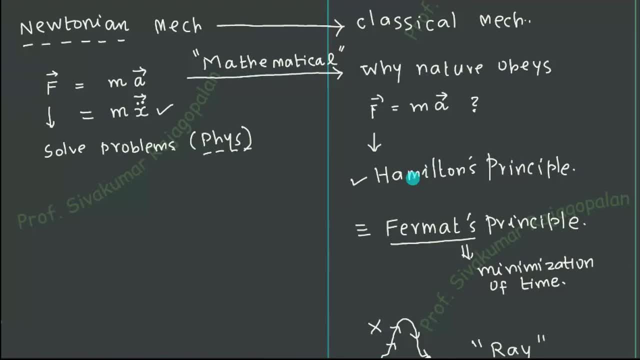 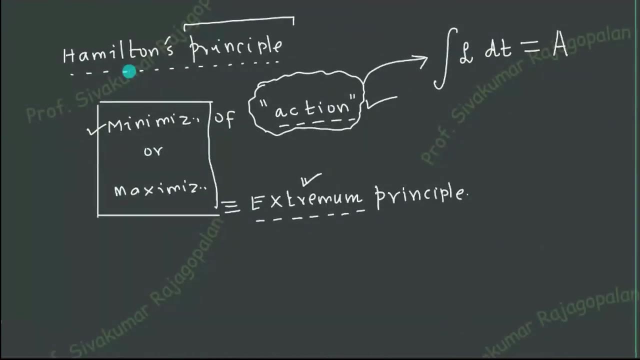 behaving in such a way that certain minimization or maximization always takes place. because of that reason, this equation f equal to ma emerges out, that's. that's what is the answer. so question is clear and answer is clear. so the answer is that: uh, the answer is very clear. the answer is that. 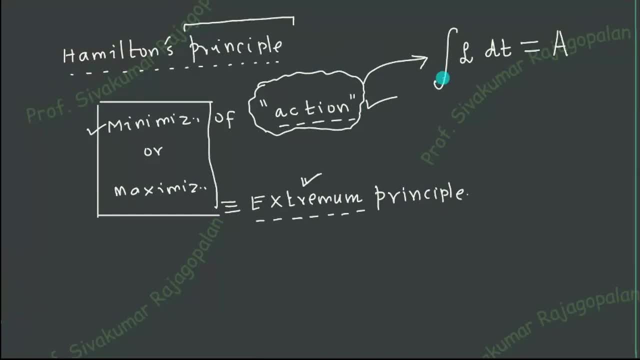 a mechanical system, we will call it as a dynamical system. okay, usually mechanical system means, you know, we call it static system or dynamic, right? if you are considering some water in the dam, okay, the dam, you have the water. right, that water is not going to move, so we consider it as an example of 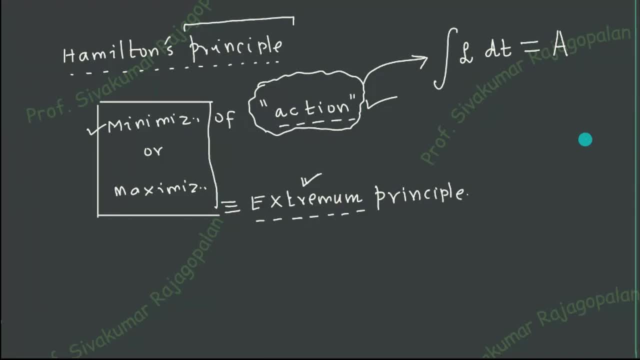 a static system and which is a mechanical system, so we can calculate what is the potential energy stored in water etc. which is not at all moving. so we say it is statics. but right now for statics we don't have the Hamilton's principle, nothing is required. 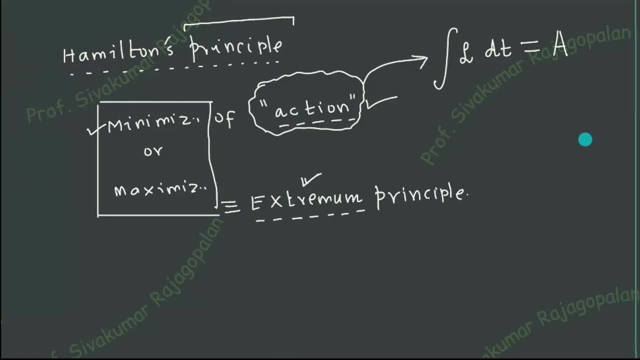 for statics the situation is much more simple. we don't require the Hamilton's principle, and Hamilton principle is required only for systems that are in motion. so systems in motion means we say only dynamics. right, therefore, instead of saying mechanical system, we will say dynamical system. so therefore, now the now we are, we can, we can now, uh, make a statement like this: 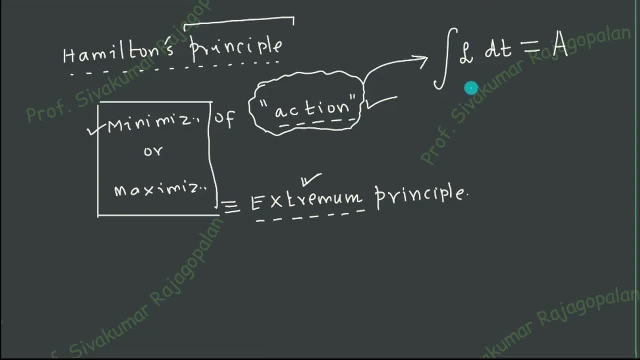 a dynamical system will behave such a way that the integral of the Lagrangian times- the time happens to be a minimum, minimum is most of the time- is valid. So we can use it. but if you want to be more, more accurate, you use the word extremum. So let me therefore repeat it: a dynamical 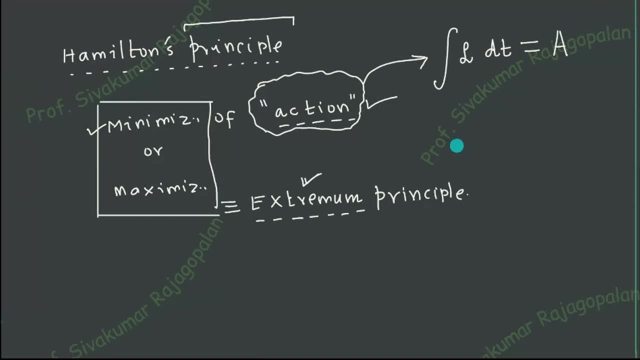 system will evolve in such a way that the integral of the Lagrangian times, dt, is an extremum. that is all. So this kind of statement that I have written down, or whatever I said Now, is this statement what is known as Hamilton's principle. 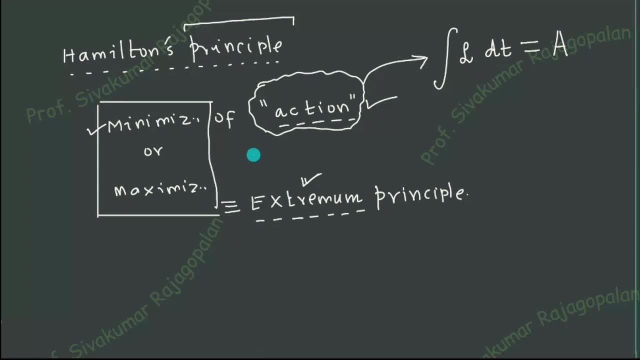 So it depends on the English that you are going to write down. Yeah, this is fine. Okay, so I have tried to explain this with a, the simplest to possible English, with a minimum wordings, and the and then the traditional books. you will see an equivalent statement. okay, so when you are, when you are going to use the equivalent, 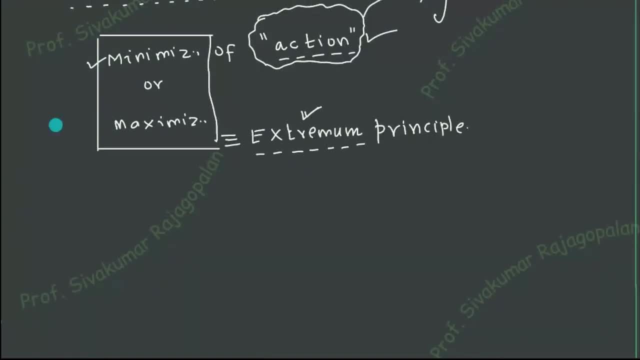 statement. let me therefore use the word here. I'll write a word. here. we're going to see a dynamical system, so that particular terminology is very important, so I am writing down. so, instead of saying a simple mechanical system, we will use the word dynamical system, which. 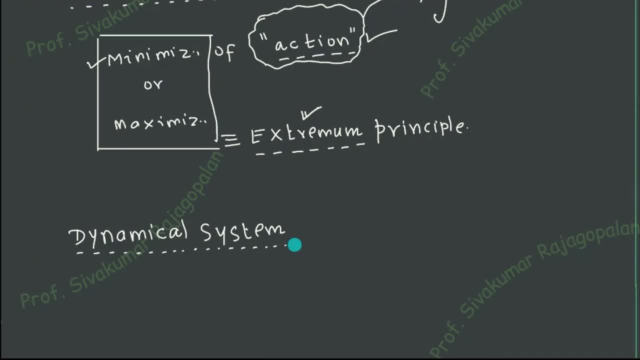 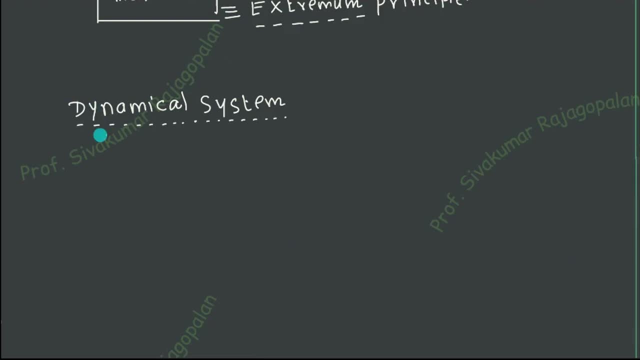 means that we no way we are talking about any kind of static situation. that is the meaning. we are excluding all statics. so in such a, in such a situation, you have to understand one thing. let me first of all explain what I am trying to do. I have written down this. 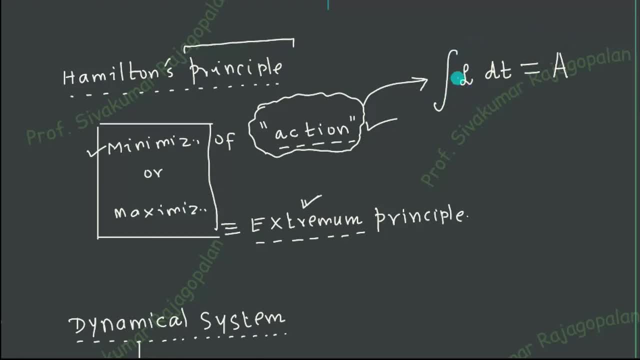 quantity right. integral of the Lagrangian times DT. but the trouble is that you have you without explaining. okay, without explaining, what is this lagrangian? i have already written the integral, isn't it? so that's why i'm trying to explain. what is that lagrangian coming there? 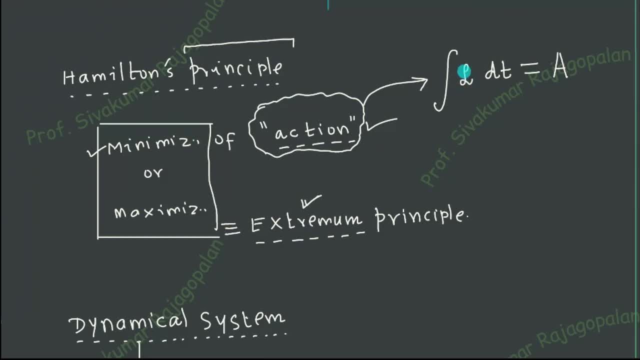 so that i will write down. but before that there is nothing to worry. it's just a function. so it is like, mathematically speaking, something like f of x- any function is given, you know how to integrate, right, it's like that: some function, that's all about it, and we will see. what is this. 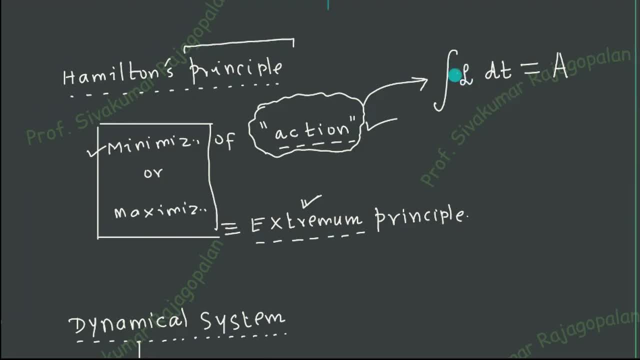 function. so there is nothing much to worry about here. we will give you, we will provide you a function here and with respect to the time you can integrate, and then, of course, you can put the limits. of course you know why the limit will come here, you see, so there is a point here and there. 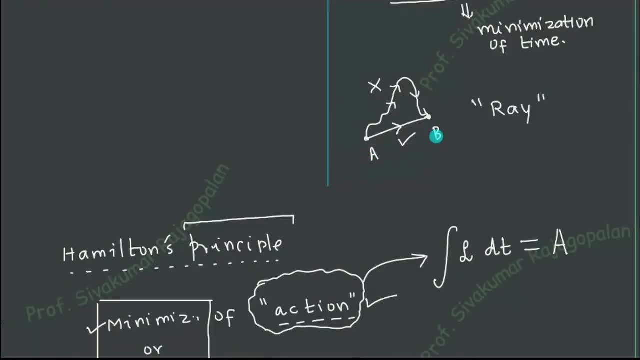 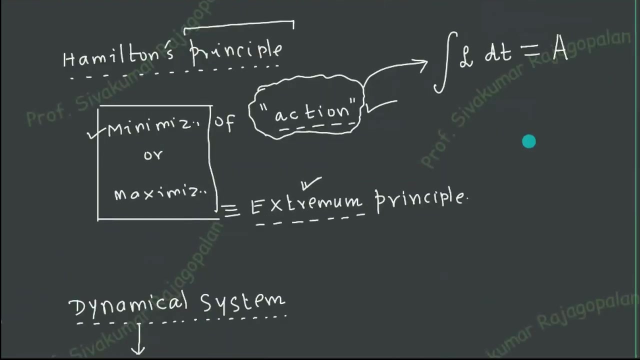 is a point b, which means that it's a starting point and then some ending point, right? so in the case of the mechanics, it is equivalent: you start an experiment at particular time and then you finish the experiment at another time. so therefore, what happens is this integral has to come with appropriate time, t1 to t2, so that 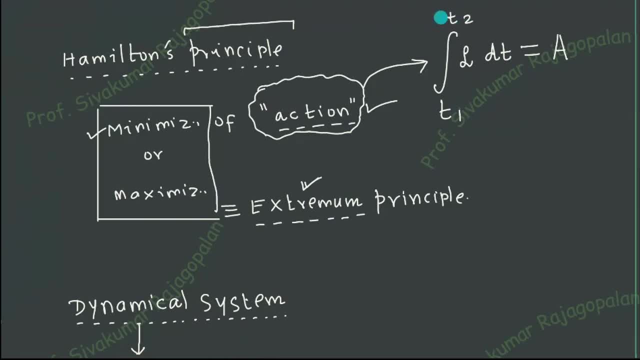 will naturally come, because you can easily understand that this has to be evaluated according to this, so that time will be eliminated in the integration and whatever left out is a quantity that is independent of time. that point should be clear to you. only if you substitute the numbers for time, time will disappear. that is a that is a general. 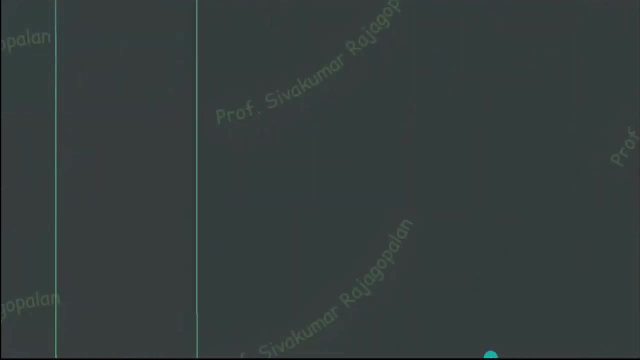 information about the definite integral, but it is not very difficult. let me therefore show you here integral of t dt. what will happen, integral of t dt if we evaluate? you know that t square by 2, but remember, t square by 2 is a function of time. function of time means what: it depends on: time. 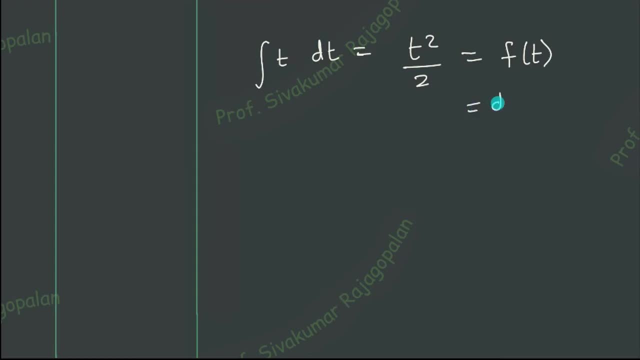 that is the meaning. f of t means what that means: it depends on time. that is the meaning. So therefore, this is the situation. now consider another example: integral 1 to 2, t, dt. now we evaluate this. this is t square by 2. now you substitute the limits of 1, 2. 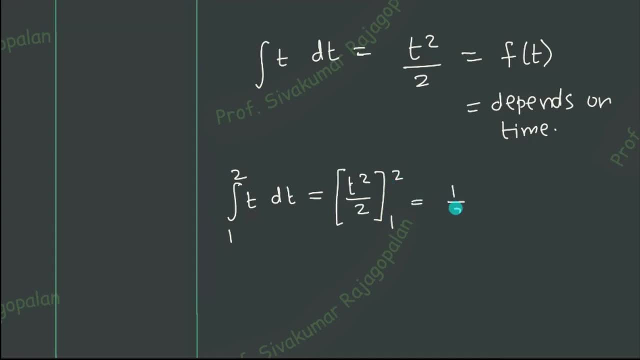 then what will happen? So 1 by 2 is common. then if I take 2 square minus 1 square, 1 square by 2, ok, so how much is that? 2 square is 4 right, 4 minus 1, 3, 3 by 2.. Now you can substitute the limits of limits 1, 2. another common arguing is that integral 1, two, 2, própria rendite power, dt should be 1 upon z squared. Now, if we take 2 square minus 1 square, ok, so how much is that 2 square is 4 right, 4 minus 1, 3. So DT to this expression of 1 by 2, now there are 10 cubed 2 squared. so now we can simply write down everyone as 3 divided by 2اد, and so we can substitute the limits one as well. 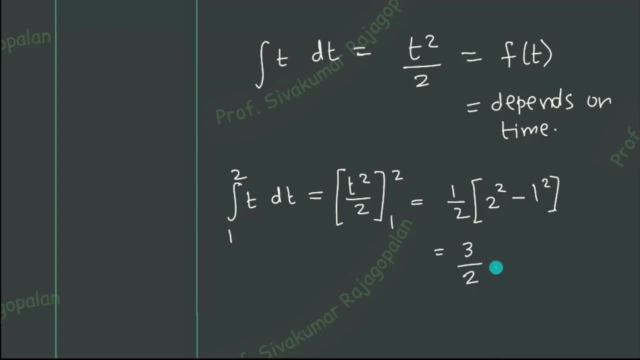 tell me whether 3 by 2 is a function of time. that is the point. so this is not a function of time. so the here it is depending on time. in this case it does not depend on time. that is very important. so this is the example of a definite integral. the first one is an example of an indefinite integral. 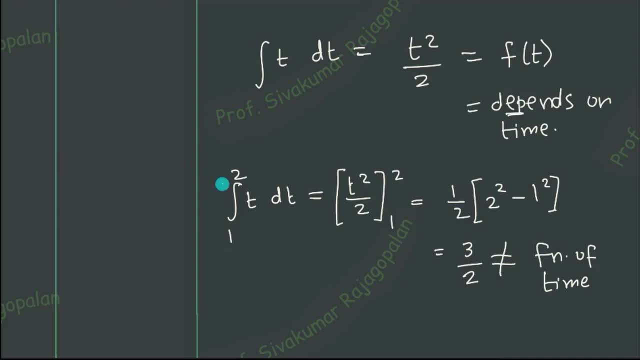 so the point to be noted is that whenever you are going to use definite integral, that means there are some limits, are there? what will happen is that particular variable will disappear. which particular variable will disappear this time? dt, is there right? so t equal to 1 to t equal to 2. 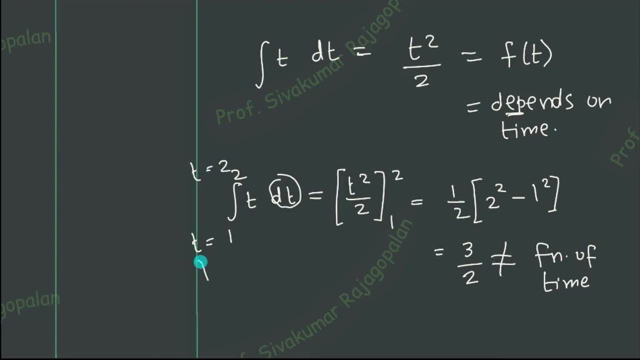 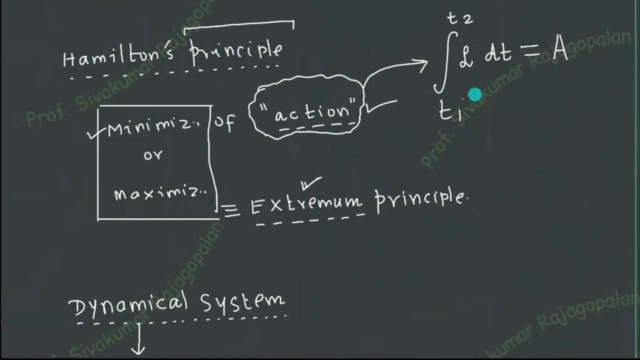 therefore that particular t will disappear, this t will disappear. so that is the property of the integration and therefore, now you come back here, now you come back and then ask the question: okay, we have written nicely in integral: t 1 to t 2, etc. You ask the question whether the action depends on time. 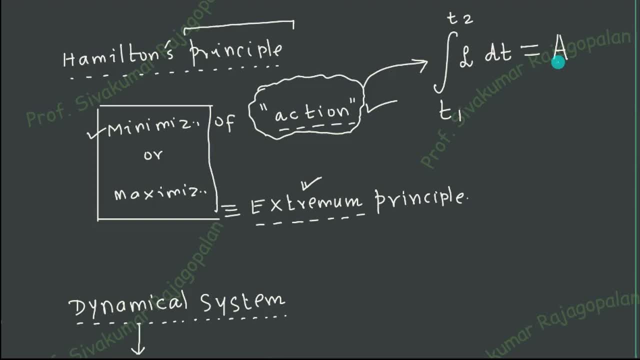 or not. The answer is: capital A does not depend on time. Why? Because there is a definite integral. I already substituted t 1 and t 2. all the time will disappear. So that is the point. So this, this quantity, is going to be an independent of time. that is the point Now. let us now come back. 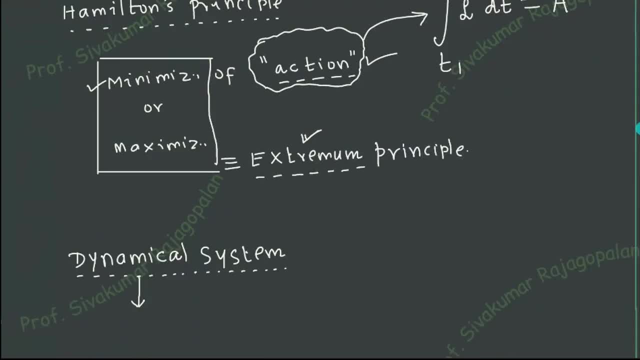 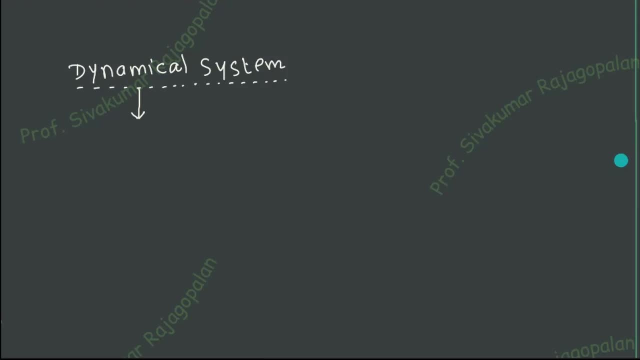 to the Lagrangian, So I will try to explain that. So what is that we are going to do is that we are going to consider only dynamical system, and dynamical system means a system which is going to move Because of this reason. what happens is: you can easily understand something. 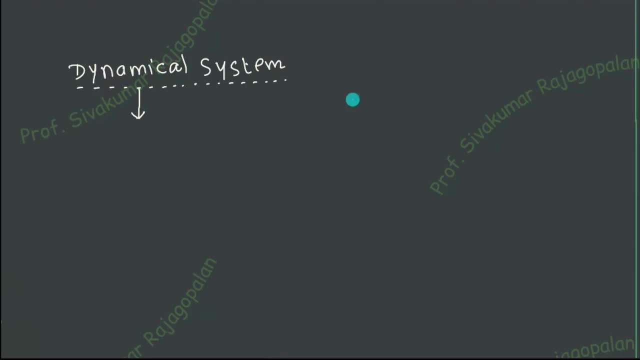 nicely So. let me therefore give an example: Consider this particular floor, whatever it is floor or horizontal line, and then you consider a ball running over there. So you consider a ball here and this ball is going to move. You have given a initial push. 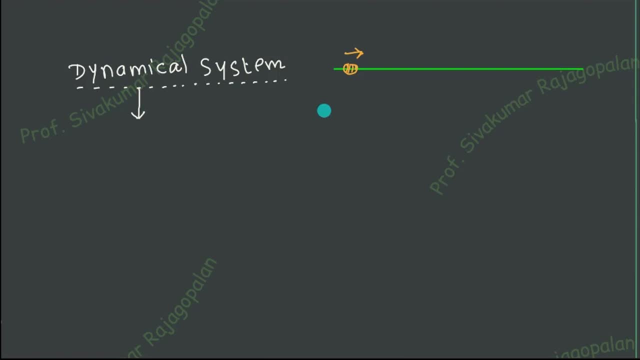 or initial velocity. So the ball is going to move. So what happens is that I am going to have a stop block with me and then I can measure what is happening at various times: t equal to 1, t equal to 2, etc. That means t equal to 1 is not the position, So position has to be measured. 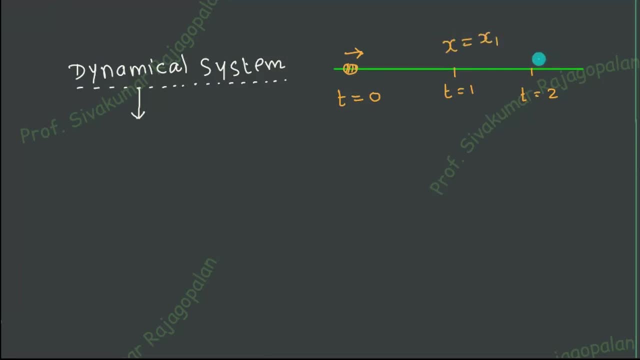 here I will write down that this is x equal to x 1.. This position is x equal to x 2.. And, of course, this particular position will be: x is equal to x. naught, You are going to start. t equal to 0, t equal to 1, t equal to 2 is time In your stop block it will show you that t equal 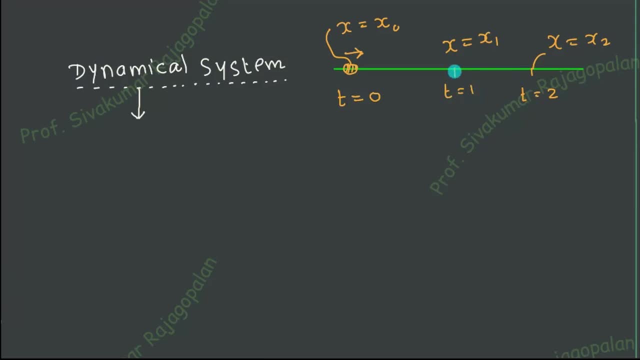 to 1 second. When t equal to 1 second, this ball will come here. If you wait for one more second, the ball will come here. That is the meaning. So that is nice. But then what happens is that, after understanding this, your experimental data will be like this With respect to the 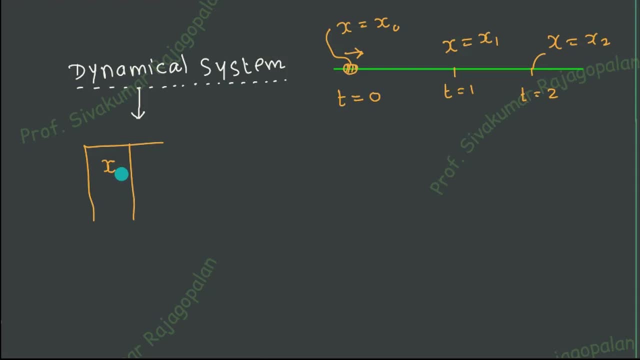 I should first write time, because that is an independent variable, So that should be the first variable, Then the x will come here and then. So this will be the tabular column that you will be filling In an experiment. that is what you do. At various times you measure the. 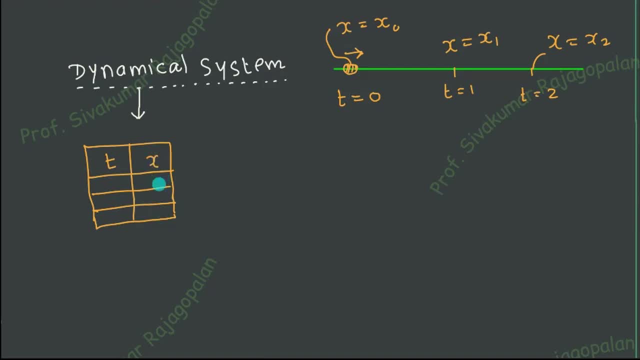 position and then make the tabular column. Now from this, what happens is that this data is not enough. So this point is important. So once you have this, you can do additional calculation like what is dx by dt. This can be done additionally. Once you have this data, you can calculate. 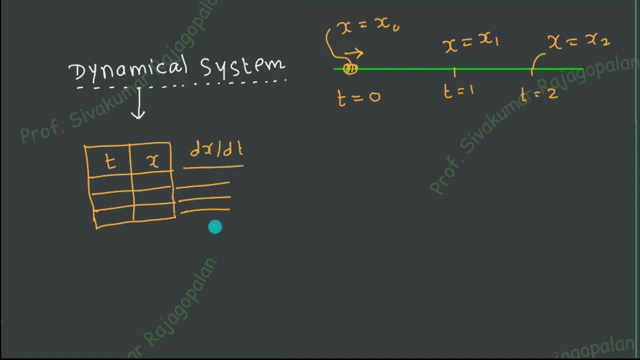 dx by dt. So, therefore, what happens is that we have three quantities: are there? One is time, One is time. The second one is the position. The third one is the velocity. Instead of saying what is the velocity, So we will sentence that kind of function And we are going to 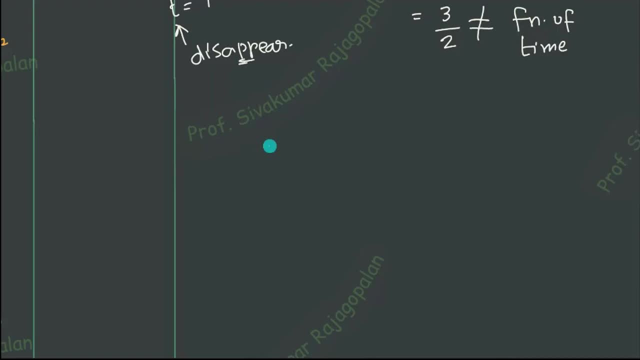 use this at this particular moment And to, for instance, we are going to put this particular function: Now, once we put this one thing from here, we are going to call it x, But notice that we are adding here function x here first. So under function x, Here you have one comma, one comma, one comma and enter. 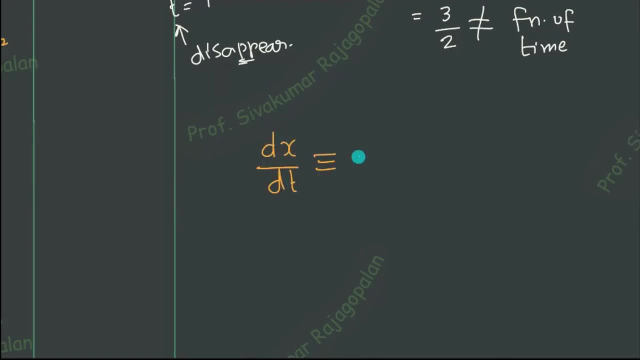 here the parameter. And then when you add this, notamment by comma, then this is an additional point to be taken from the variable size. In this case we, inside the example, we recommend 2, Stanford, and note the value of 1 and 2.. And so野r 2. this form can be spell out whatever2n half. So now you know differences. 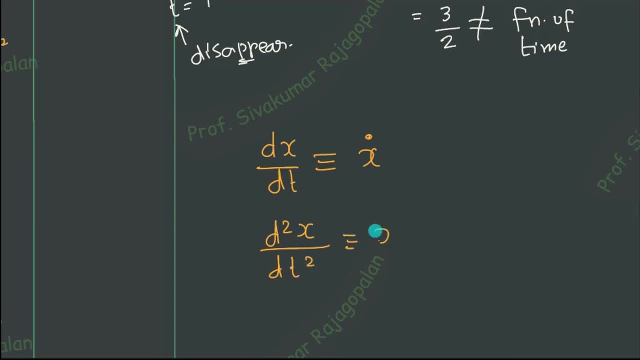 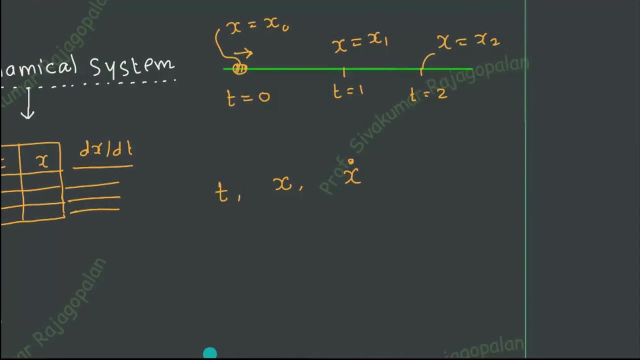 in every number of numbers and you can compute two up to one. Now, here, here you see, 4x 13, the single dot and double dot notation we will be using. so this is the we say velocity and acceleration, so based on this notation. so here, what do you understand from this experiment is: 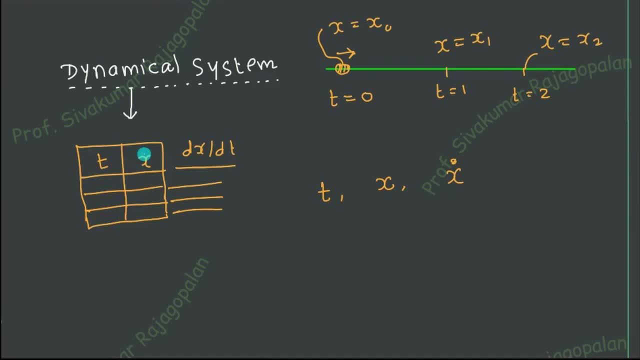 that with respect to time i measure the position. after that i can calculate the x dot. that is one option. the second option is there. second option is: if you are going to consider the pendulum, you consider a different experiment. if you are going to consider a pendulum experiment, 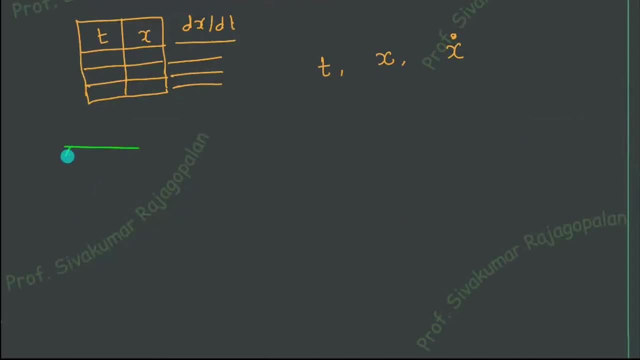 okay, you consider, i'll, i'll show like this. so you consider some kind of a pendulum like this and then put it like that and it is oscillating now. so in this case, what will happen? you have to think. in this case, what happens is: you can. 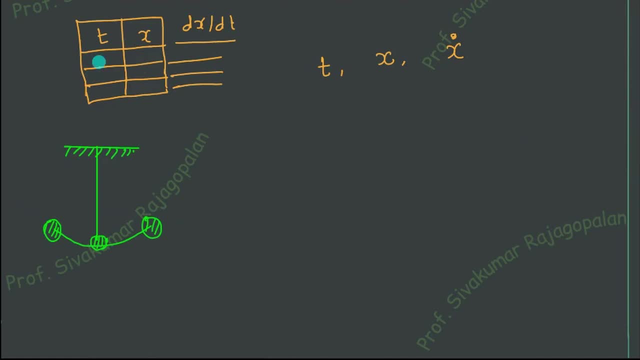 not write down a table or column like this. it's not possible. you can try with respect to the various time. what happens is writing down the different position is not easy, because this is making an angular right: you, you don't have a position, you can't measure. 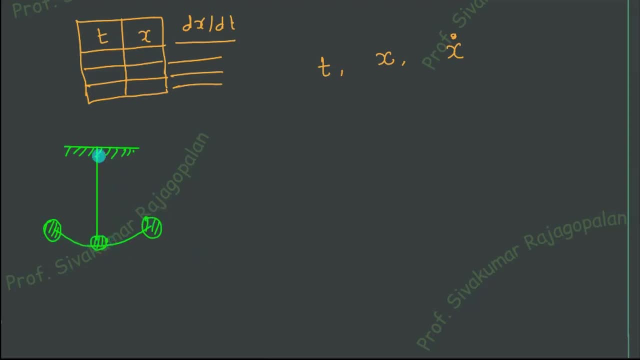 x-axis. what is the value? because it is moving like this. actually, what you have to measure is you have to measure the angle. so measuring the angle theta will be difficult as it is oscillating. okay, suddenly you cannot say 21 degrees, you can't be 43 degree, 23 degree, 7 degree, like that. you can't measure. so, therefore, what happens? 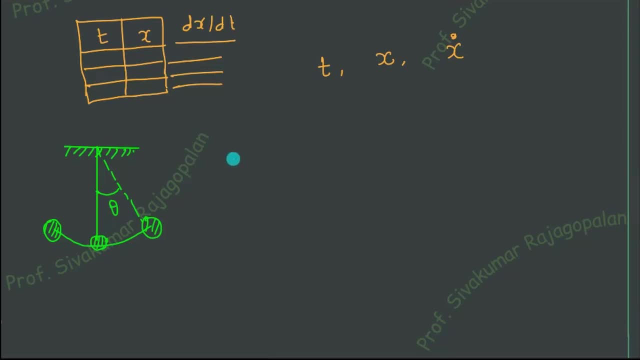 is in such a situation. what what people generally do is that, at various times, what happens is you measure the position, for example, some selected position, uh, with theta. okay, now i will write down the better. the symbol should be better, because the position is not x, comma, y, comma, z. right now it is theta, so i'll say theta. 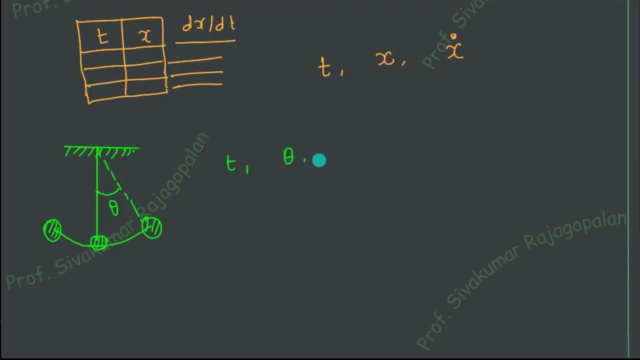 so when you are starting the experiment, what happens is: i will be knowing theta dot. now this point should be clear to you. you must be able to agree where from the three numbers are coming, otherwise you cannot understand lagrangian. this is important. you, when you are performing this experiment, what is the data available to you? that is the question. answer is: 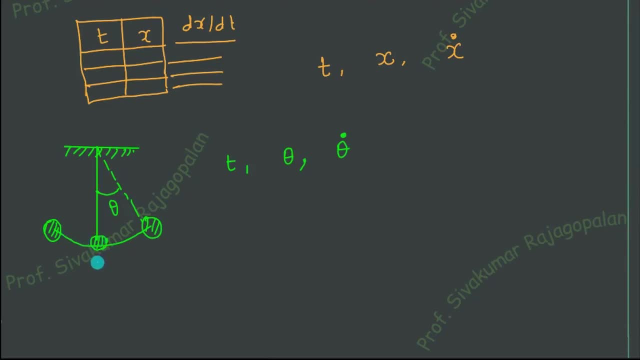 this. the answer is: at time t equal to 0. so this is the time t equal to 0, at time t equal to 0. my theta dot is 0 and theta is not equal to 0. do you agree for this? this is how you start the. 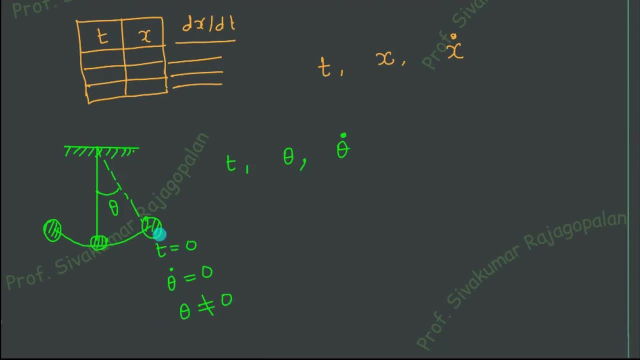 experiment. if you have done the simple pendulum experiment, you remember how you do. you pull the bob and hold it. you have to hold it. holding means what theta dot is 0, that means it is not moving. and when you are holding angle is not 0 degree, maybe it is 10 degree, 8 degree, 11 degree. whatever it is, some number is there and 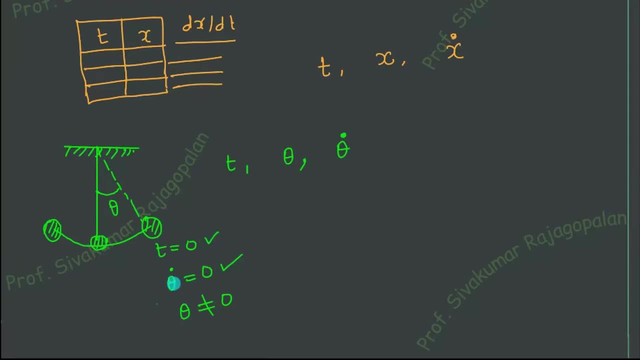 your stop block will show 0. the bob is not moving, therefore 0, and it is at an angle 10 degrees. therefore, that is not 0.. so how many numbers do you have, or what are? what is the data that you have? i have t, comma, theta, comma, theta dot in a simple pendulum experiment. in the case of the previous, 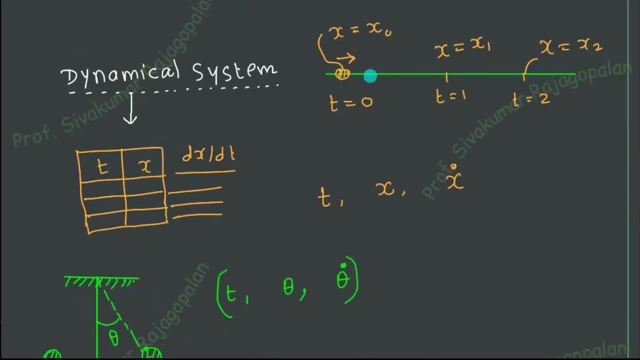 experiment where you see that a particular ball is allowed to roll. you can. you can allow to roll on a horizontal plane, inclined plane, anything is okay, but ultimately, what is the data that you have? the data that i'll be having is time can be there. either you can have x and x dot or you can measure. 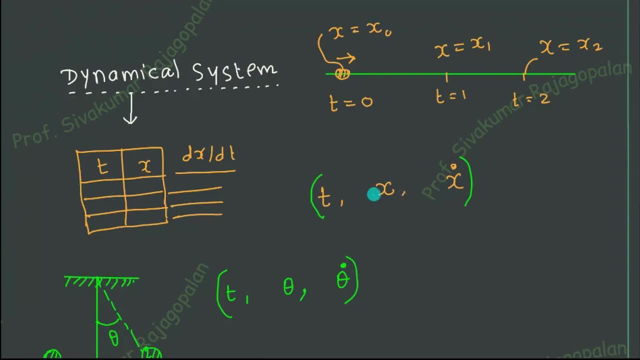 all the x and calculate x dot. so what happens is in many of that systems, so these are two of the systems. in many of the dynamical systems what happens is we will be requiring all the x and x dot. we will be having the set of numbers- time, comma, position, comma, velocity. so 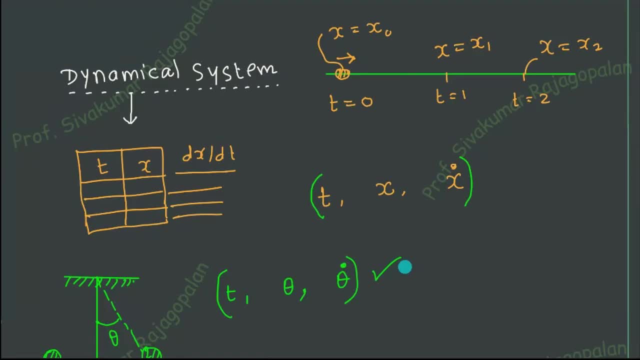 this is what you understand from your experimental knowledge. any experiment you take, you can always find out time position and the position time derivative. position time derivative is called velocity. so whether it is, whether it is linear velocity, X dot, or angular velocity, theta dot, that's not a problem. 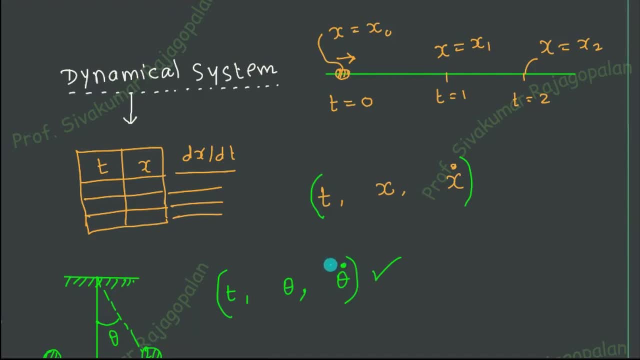 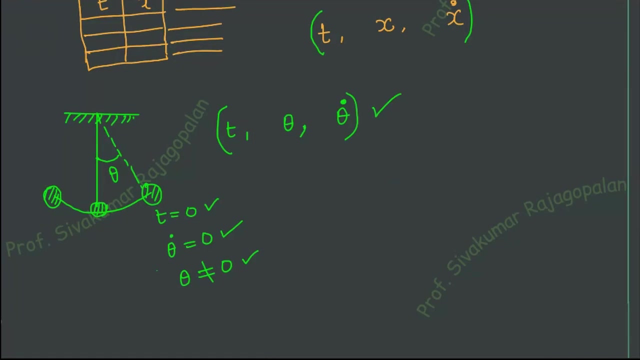 but? but there is some position and there is some velocity. that is a point that you should remember. so there are three variables are coming. remember that there are three variables are coming. so, therefore, what happens is now, you know, now comes the important point. so what happens is that we are going to have okay. 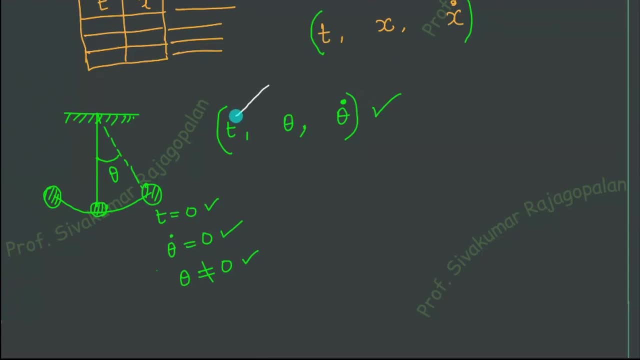 so you have TT, right? even though I have written in a different place, I will put arrow. so there is a time here. there is a time here, right? so therefore, now I will write down like this in a box: so you are going to have three quantities. okay, we are going to have. 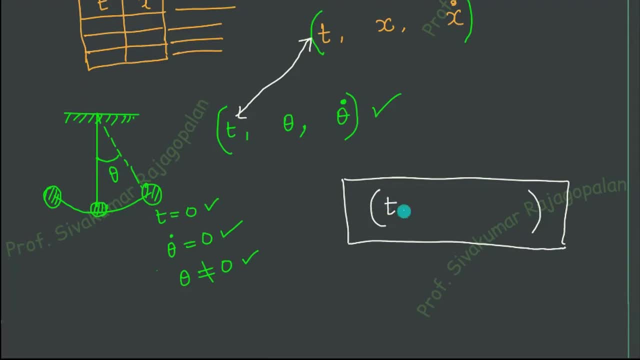 three quantities. one of the quantities is time T. I will write down T. that is common, so it is not changing. so therefore I'll write down second quantity: in first case it is X, the second case it is theta. X and the theta are not same because X can be in meters. right, you can measure meter centimeter. 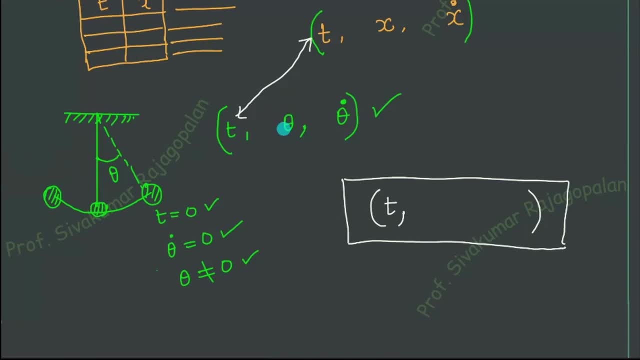 but theta cannot be measured in centimeter, so typically it means that Taaaaaaaaaaa, that something is different. you can't say always distance, okay, using the word distance is not at all correct for theta. so this gives you an indication that sometimes position may come, sometimes angle. 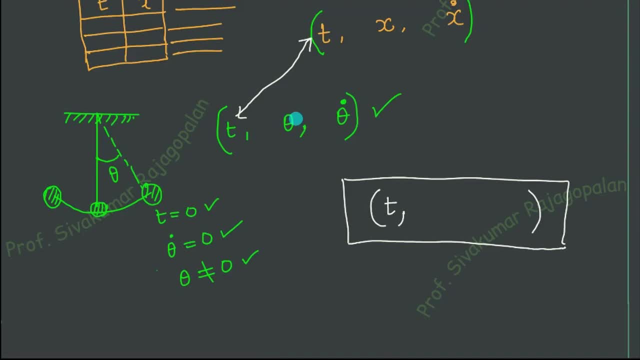 may come, sometimes it may be different, we do not know. so therefore, what happens is people have an idea that why shall we write x here or shall we write theta? people thought that, okay, let us not write both of them, we will write a general symbol, q. you understand what is the q? q is a general. 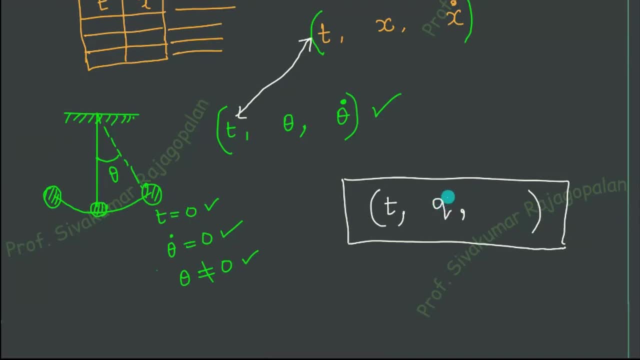 symbol, general symbol means q is nothing but position in that experiment. q is nothing but theta in the simple pendulum experiment and q can be something else in another experiment. that is an idea. so q, what is meant by q here is q is called generalized, coordinate, generalized. 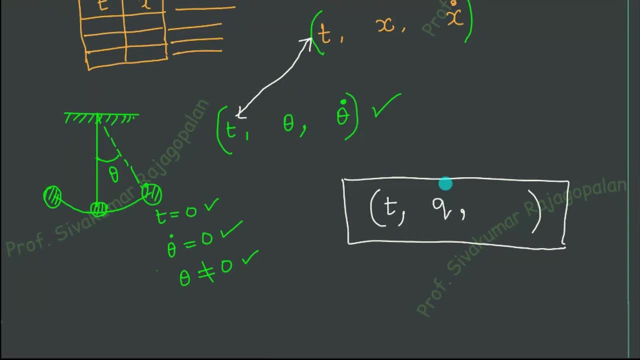 means. we don't say that it has the dimension of meter, we don't say that it has dimension of radians. we don't say anything. we do not know what it. it can be anything that is called general, so it is generalized. and if that is the situation, then what will happen to that theta dot? so here theta dot is. 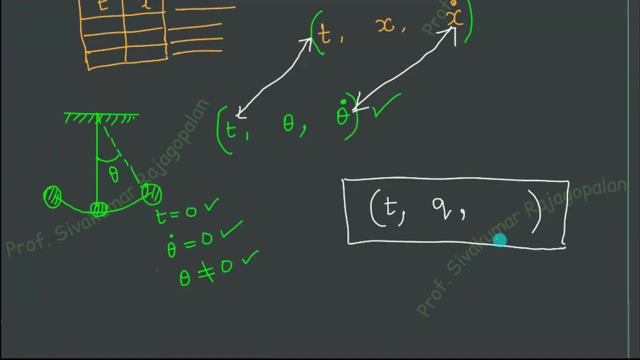 there and here you have an x dot. so what shall i write here? so that should be the time derivative of the position. so therefore it becomes q dot. so if q represent the position, q dot represent the velocity. we don't use the word angular velocity, we don't use the word linear velocity, but instead we say that it is generalized velocity. because you 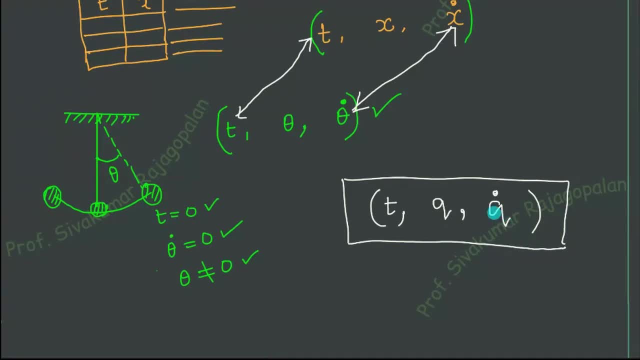 do not know what it is right. if you exactly tell me it is a, it is a simple pendulum experiment, then okay. if you tell that it is simple pendulum experiment, i will say that it is angular velocity. if you particularly tell that it is moving in an horizontal plane, then i will say that it is a. 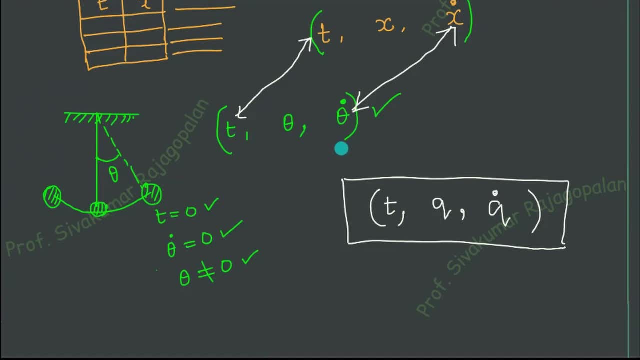 linear velocity. until that, until that means when i do not know what kind of physical system i am explaining, i also do not know whether it is linear or angular, and therefore it is better to say generalized. and that is the reason why we have this kind of coordinates, and this is what is known. 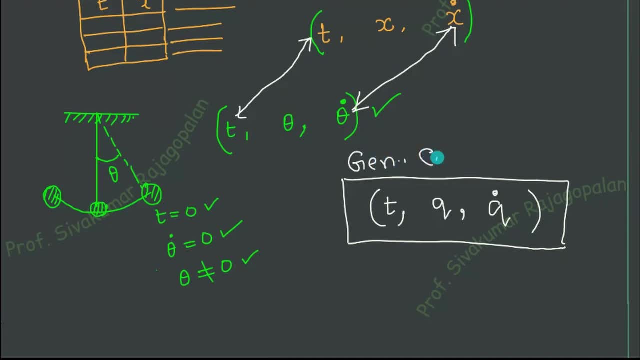 as generalized coordinates. i will say: this is generalized coordinates and generalized velocity. so you have this, of course, for time we don't. there is no confusion. there is nothing like generalized time. that is not there. time is time only. so in any of the experiment, therefore, the problem comes only. 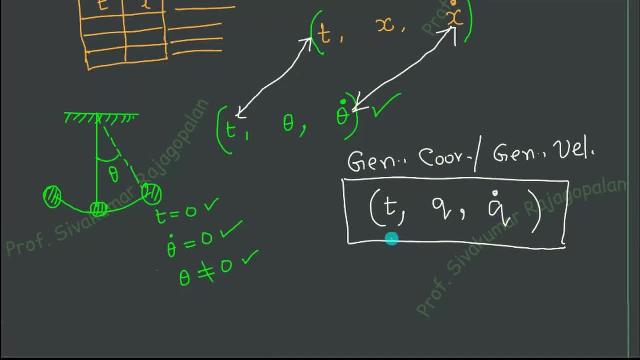 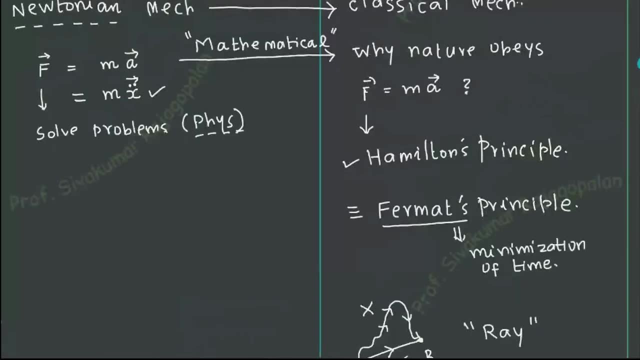 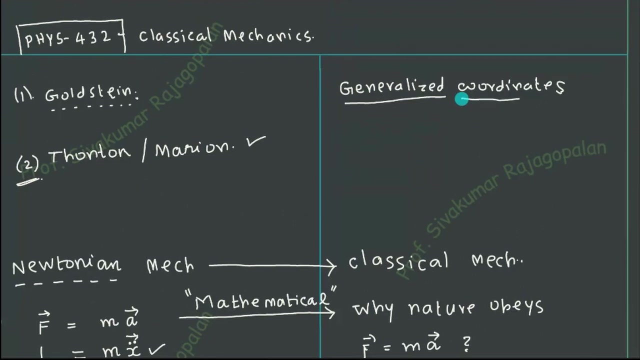 for the position and the velocities and remember that that is how it looks like. and if you go back, let us start. let us go to the beginning of today's class. you remember what did i write here? it is there. so i told you that the starting point for the 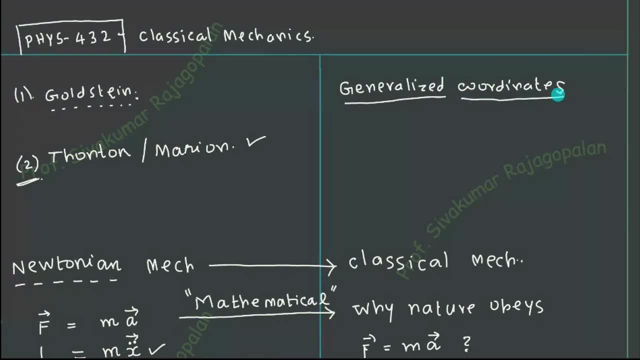 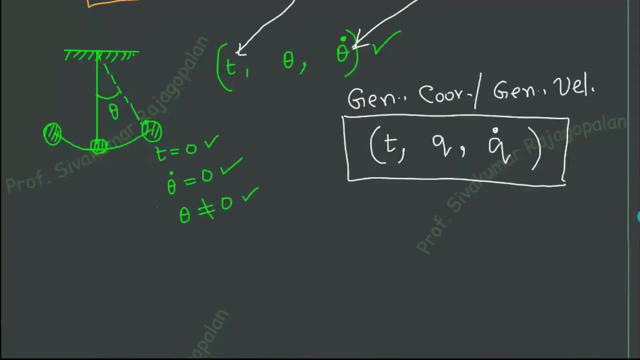 classical mechanics would be understanding the generalized coordinates and generalized velocity, and then then we can think about. so we need the idea about the generalized coordinate. that is what i said in the beginning of the class, and now you understand what is meant by a generalized coordinate and generalized velocity. now you understand what it is, and this is nothing but. 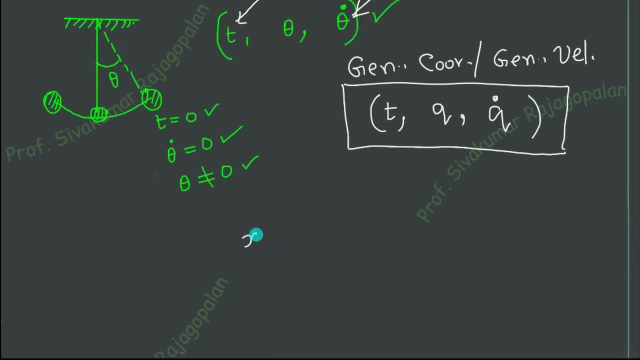 coming to, mathematically we can say three variables: x, comma, y comma, z. okay, the mathematician will say: okay, x comma, y comma is a three variables. t comma, q comma, q, dot, three variable. it's a function of three variable. so i'll say that it's a function of three variables. so, mathematicians, you can easily write down now: 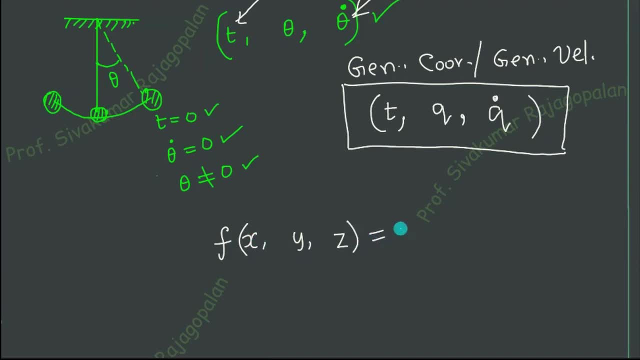 tell me an example of a function of three variables means i can easily tell: okay, x, y plus something like y z, square, plus x, y, z, anything you can write. now that function which i have written is an example of function of three variables, so any function can be written down. 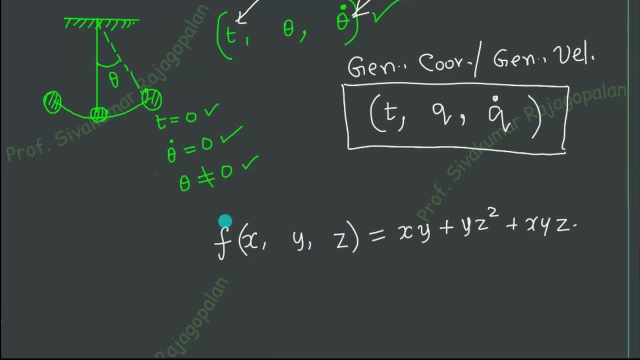 which can be a function of three variables. mathematically speaking, and now coming to the case of the classical mechanics, we are going to write down a function of three variables, where the first variable- we are going to call it by the name- q. second variable, q- dot, and the third 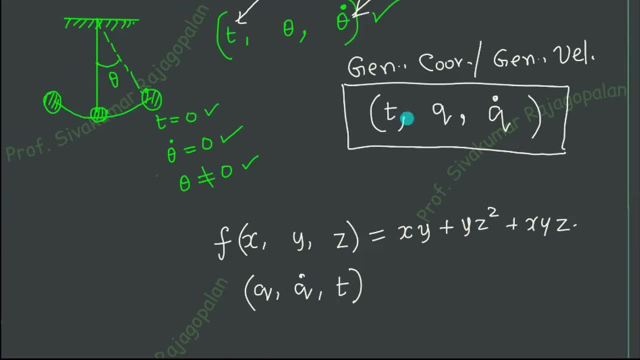 variable t, this t, q, dot q. okay, that order is only uh interchange and it is traditional to write in this order and instead of saying that it is a function of f, we can say f of, we can say g of g of x, f of x. anything can be written and in the case of the physics, what happens is we are interested. 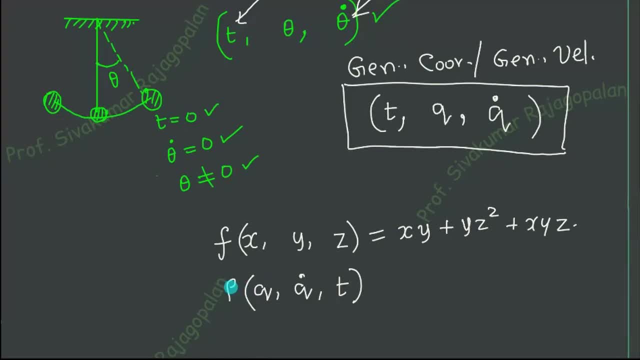 in a function which is called the lagrangian and therefore we say it is l, it can be f, only f of q comma, q, dot comma, t. fine, there is nothing wrong in that. it is a function of three variables. but actually that function is called by the name lagrangian and therefore, instead of using f, 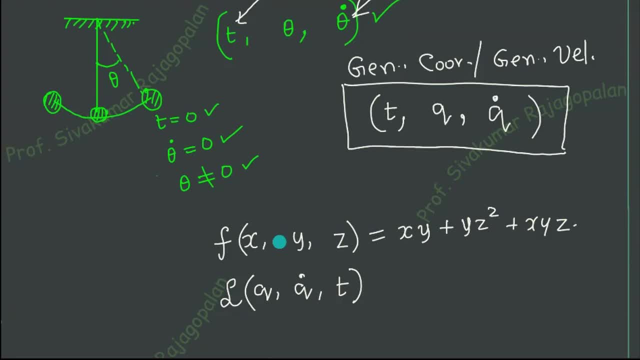 comma. instead of using g, we are using l, and this is a similar function of the lagrangian function. you can write any function here which is a function of q comma, q, dot comma, t, and this is what we are going to call by the name lagrangian. and now you understand that. if 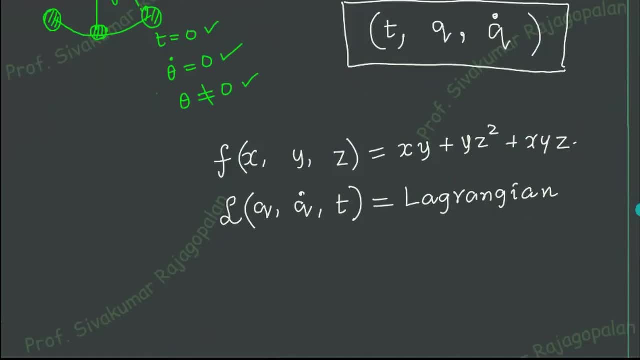 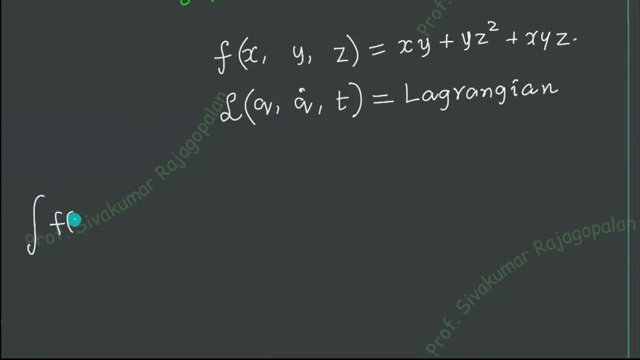 this is the lagrangian, then we can now evaluate that. if you have a function like this, you know how to integrate. if i give you a function and say that, okay, this is the function that you are having, f of x, comma, y, comma, z, evaluate with respect to d, that means you can evaluate. 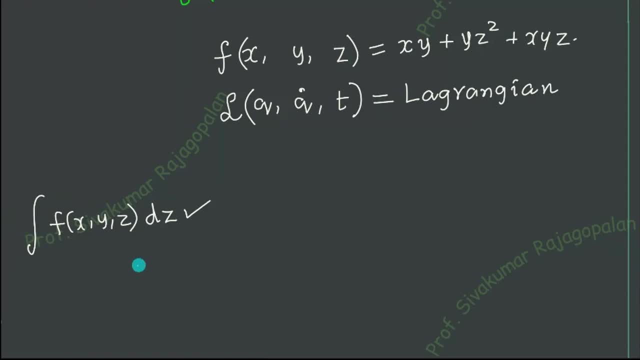 you know how to do the integration and similarly, okay, if that is the situation, similarly, you can perform the integral of q, comma q, dot, comma t, that's a dot here, comma t, and then you perform the respect to the dt and then, of course, this is from time one to time two. can you evaluate? 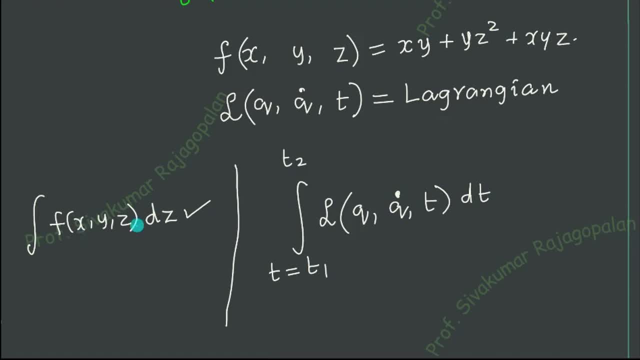 this means, yes, we can evaluate what is wrong. if you, if a function is given to you, you can evaluate. and if you evaluate and simplify- whether you're going to simplify or not, that is a different story. if, okay, if you simplify, we will call it by the name: a. 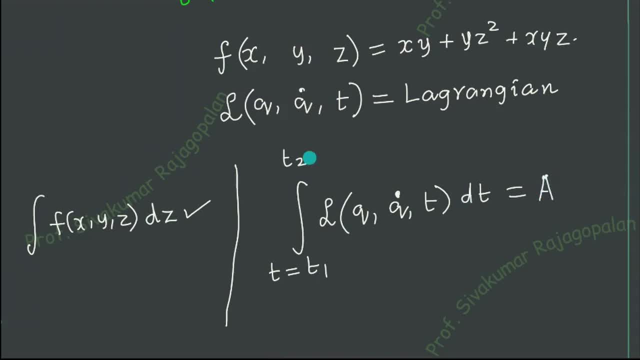 even if you don't simplify, it's okay, keep it in the form of integral. we will call that as the action. so now you understand that this is the action, action, integral, that's all. so this action integral is what is getting minimized. is what is getting minimized, okay, so, and that is called the. 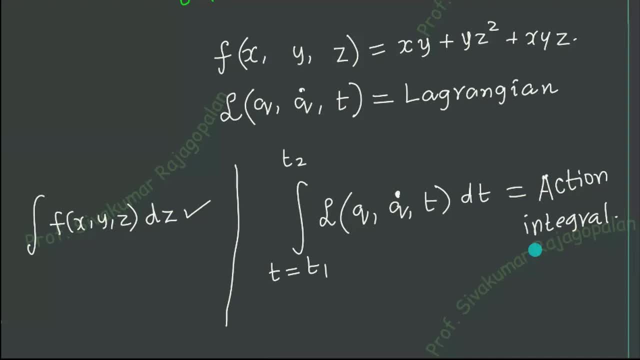 hamilton's principle. so that's all about it. and so in today's class, uh, you basically understood, uh, how you are going to make a transition from the undergraduate newtonian mechanics to the graduate level classical mechanics, and the starting point would be the hamilton's principle. that is the starting. 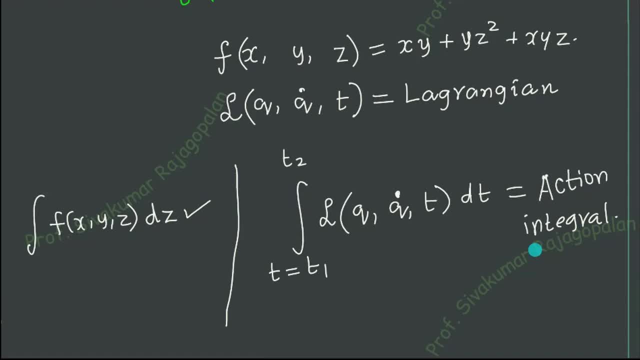 point and from here you can do some mathematics. of course, whatever we are going to do is only mathematics and we are going to see. what is that we are going to see is that, of course, we will see that this kind of principle will exactly, is going to generate f equal to me. that's the connection. so, ultimately, 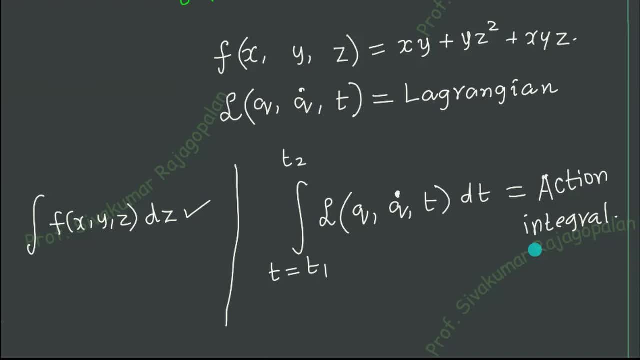 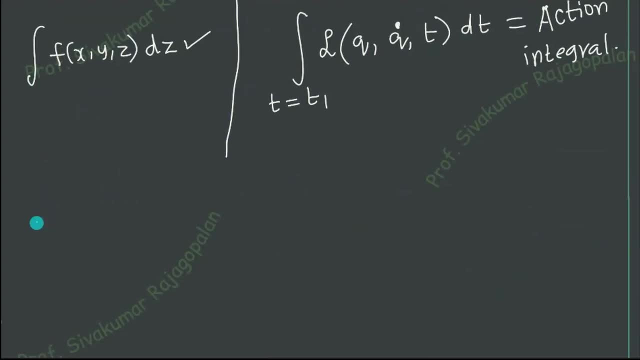 you should know what is the connection between hamilton's principle and the and the newton's law. that point should be clear to you. or, ultimately, what is happening? what is going to happen is: this is what is going to happen. i'll write down that. so the hamilton's principle. 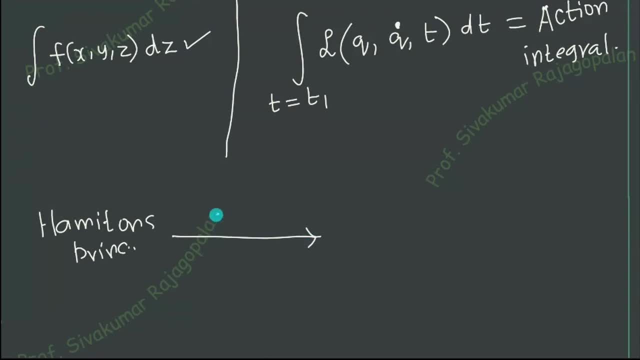 the hamilton's principle is going to generate, is going to generate f equal to me, so that, so then you'll be, uh, we will be having the answer to the question that we started. so what did we start in today's class? we asked the question: uh, on what basis? on what basis? 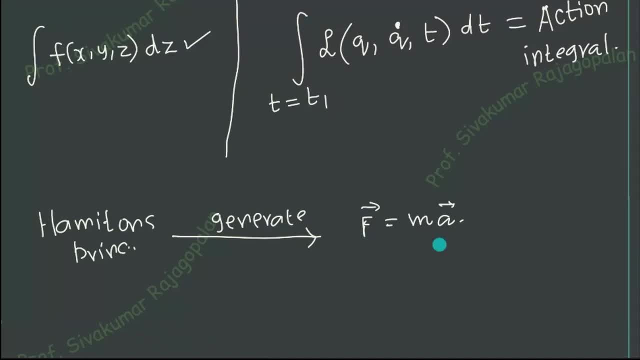 f equal to me, uh is derived. or we say that on what basis nature is uh, nature is uh behaving according to f equal to me. that is the question. the answer is that hamilton's principle is the underlying principle. that means this has to generate that. that is the meaning, that the meaning is hamilton's. 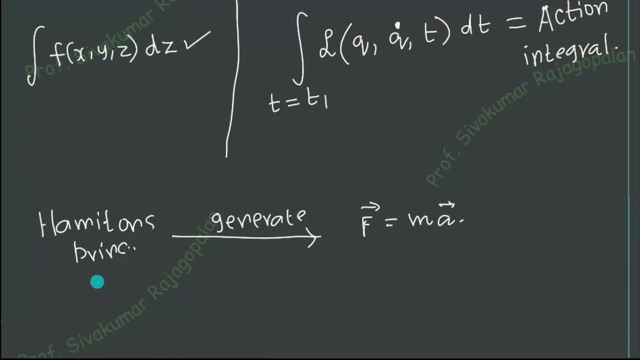 principle is going to be much, much wider principle, not limited to mechanics alone. but if you say f equal to ma, f equal to ma is very particular to a physical system in mechanics only. this is not applicable to some other topic. that is a meaning. therefore, hamilton's principle is much, much. 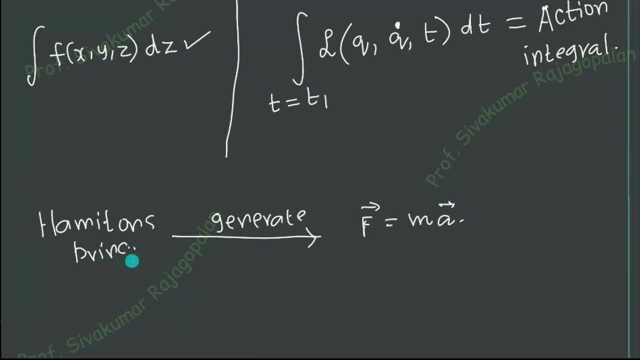 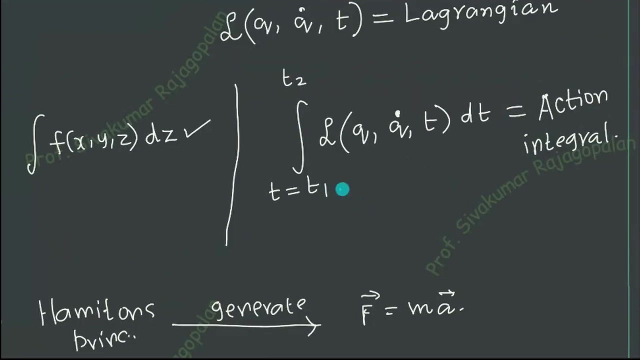 general principle rather than limited to a particular topic. so that is the overall, all conclusion. so remember that this is a very important and crucial one: why people are, why should i write the lagrangian to be a function of three variable? that three variable actually comes from the, from the experimental knowledge. okay, any given physical system you will be having 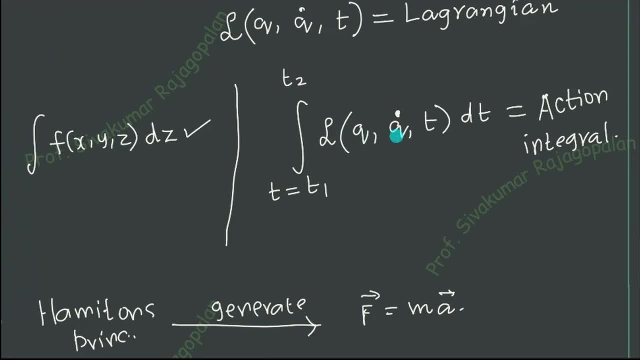 the data for time, position and velocity. that is the reason. okay, with that, we will stop and probably will see how we are going to proceed. okay, so any questions that you want before closing today's lecture, you can ask now. okay, then. so i'll close the meeting then. okay, okay, thank you. 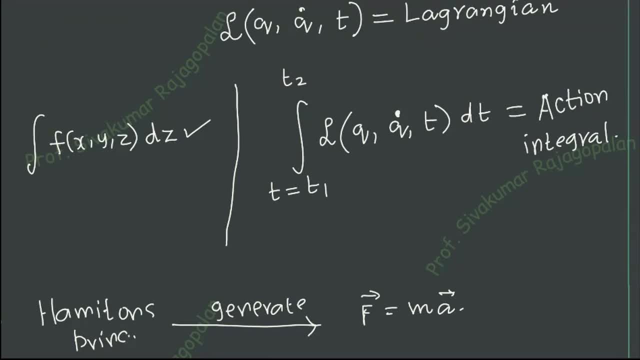